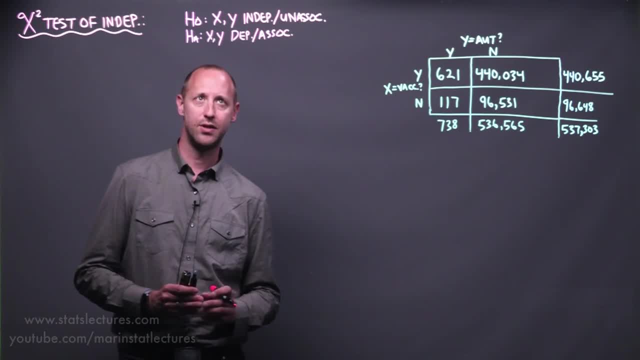 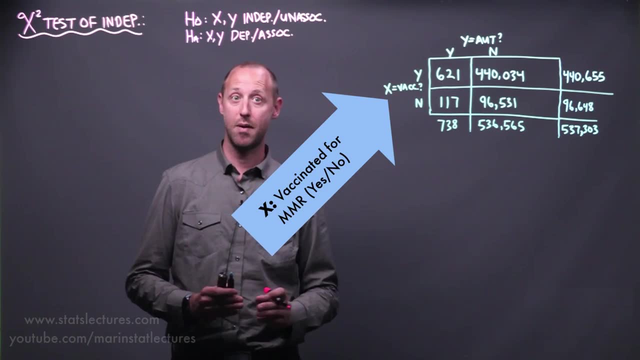 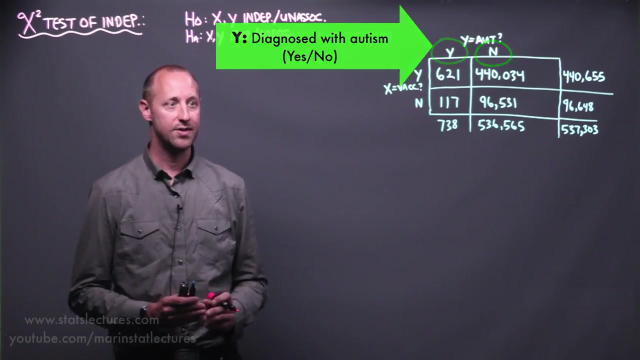 from a paper published in the New England Journal of Medicine in 2002, and it's looking at an x variable of whether or not a child was vaccinated for MMR, measles, mumps and rubella- yes or no, and whether or not they were diagnosed with autism- yes or no. And so the question here: 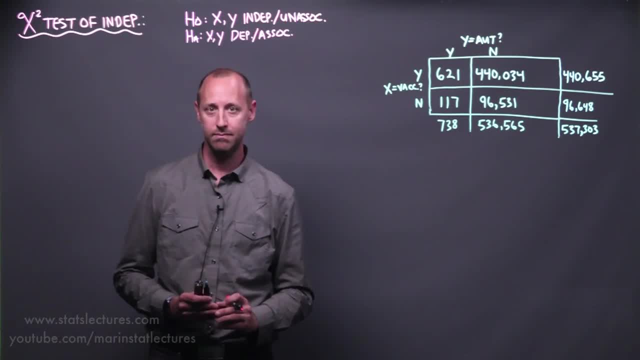 we'd like to ask is: is there any relationship between x and y? So, stating it generically, we're in a situation where we have a child who is vaccinated for MMR, measles, mumps and rubella. we're going to start with a null hypothesis that x and y are independent or unassociated. 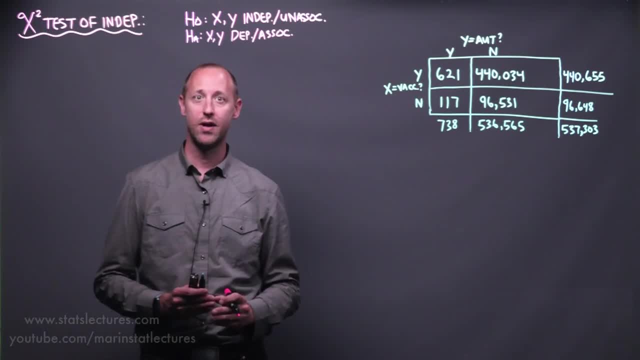 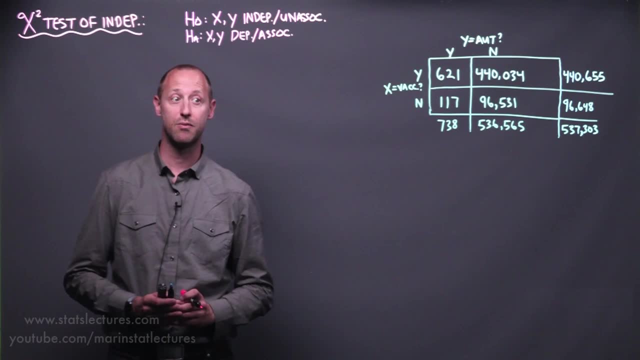 or that there is no relationship between getting vaccinated for MMR and being diagnosed with autism, and an alternative hypothesis that there is some dependency or some association or some relationship between the two. So the main kind of probabilities of interest we're going to look at, 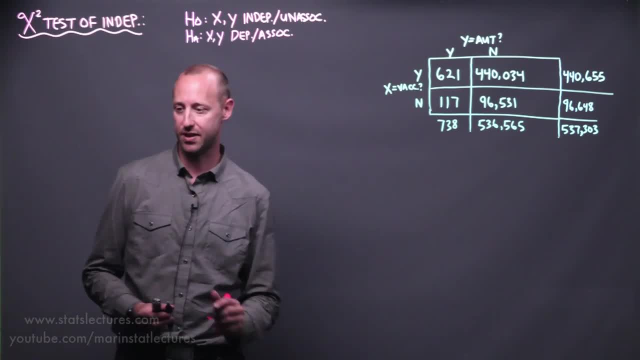 here is. we're really interested in comparing two probabilities here. The first one I'm going to label p1 hat. Okay, hat means that I'm going to have a child who is vaccinated for MMR, measles, mumps and rubella. 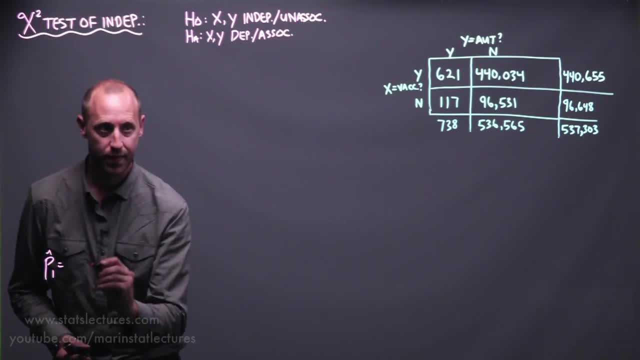 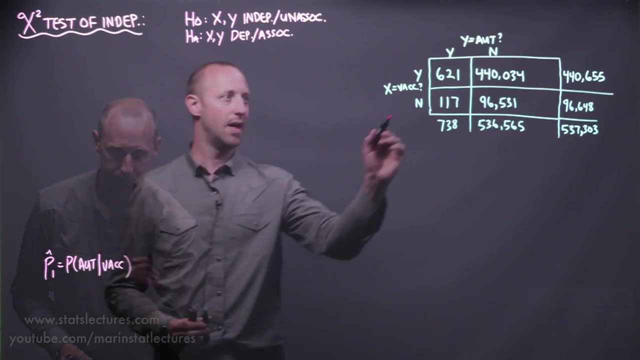 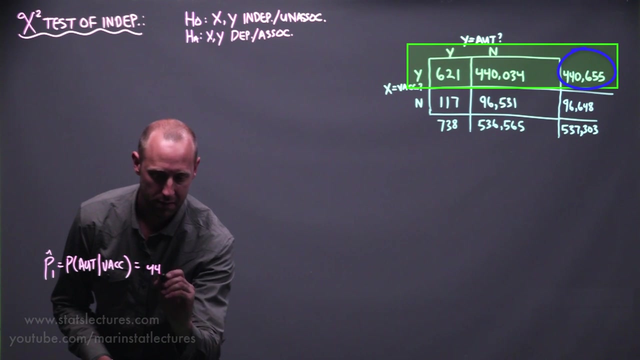 meaning it's a sample estimate from our data. What's the probability of developing autism, given that they were vaccinated, And we can see we're conditioning on this row here- Out of the 440,655 who were vaccinated, 621 were diagnosed with autism And this comes out to be 0.025.. 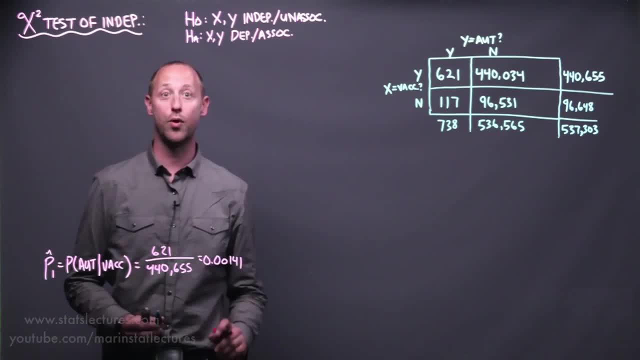 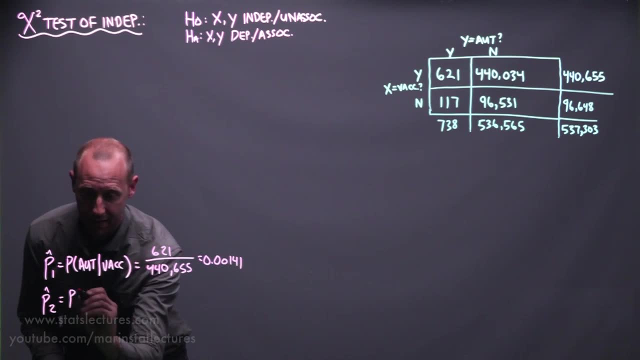 0.0141, or 0.141%, And the other probability we're going to be interested in looking at, or other proportion, is the probability of being diagnosed with autism, given that they were not vaccinated. Again, that's conditioning on this row here Out of the 96,648,. 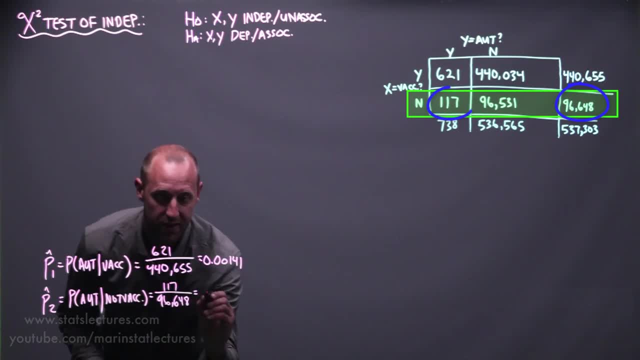 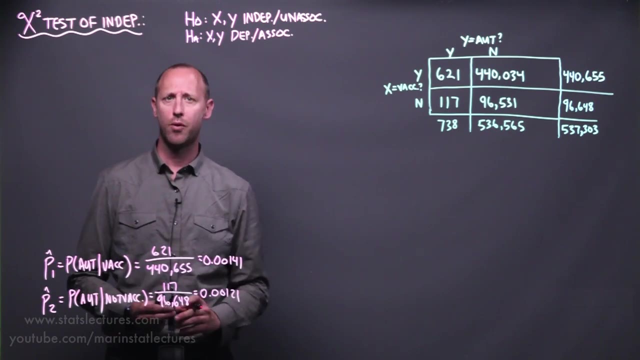 who were not vaccinated, 117 were diagnosed with autism, And this is going to come out to be 0.00121, or 0.121%. So, in some sense, these are the two proportions or probabilities that we're going to want to compare, And we're going to do it using the chi-squared test, although it's worth. 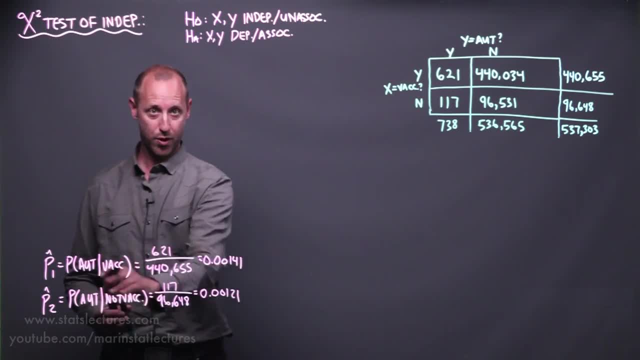 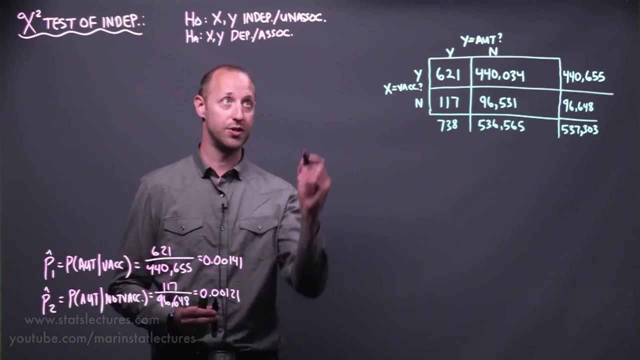 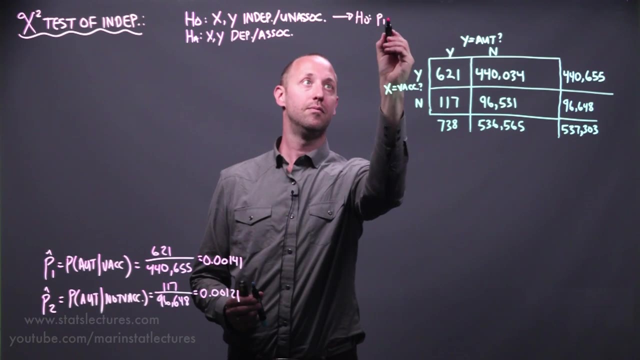 noting that often you also encounter this difference in proportions approach, making a confidence interval for the difference in two proportions or testing a hypothesis about the difference in two proportions. So we can also express the null hypothesis as being that p1 is equal to p2, right At the population level, these two proportions are equal. 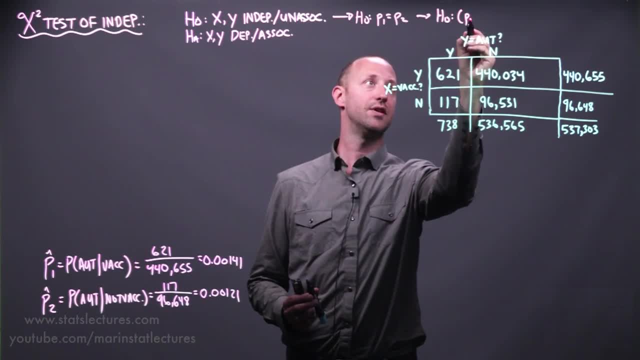 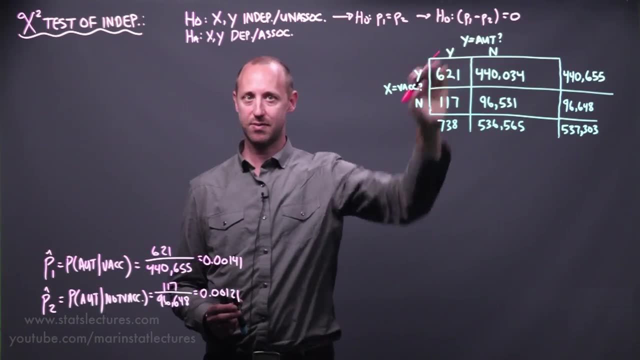 Or we can also express it that the difference in the proportions is zero, that there is no difference. And again a reminder: often we express things this way because that boils things down to having one estimate that we can look at, One estimate we're going to test. 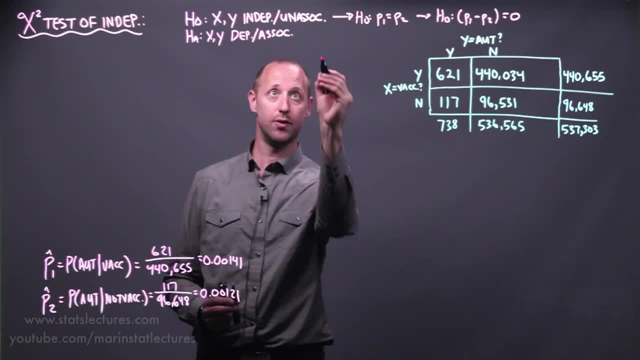 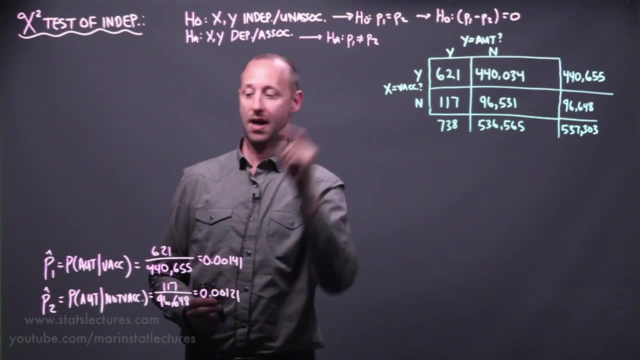 a hypothesis about one estimate we're going to build a confidence interval for, And so, similarly, we can state the alternative, that these two proportions at the population level are not equal. right, The probability of being diagnosed with autism is different for those who are. 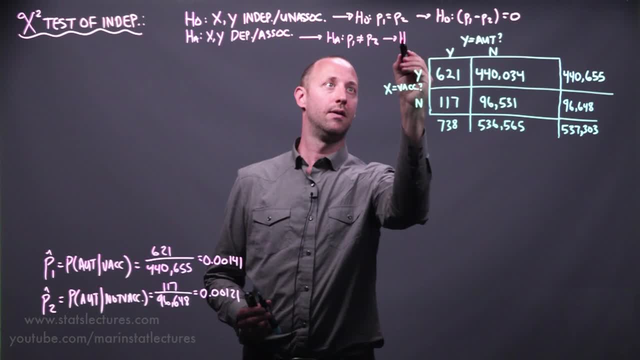 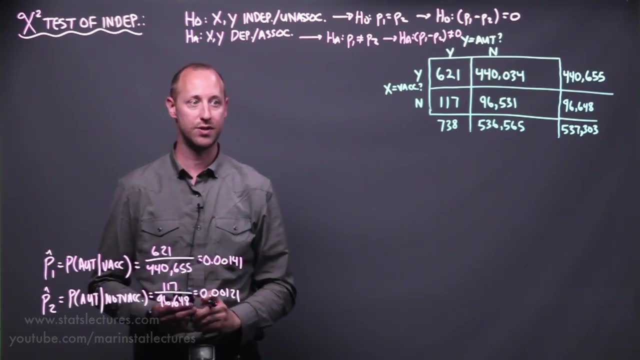 vaccinated than those who are not And, as noted, we can also state this as the difference in the two proportions is not equal to zero through using the chi-square test. but just a note, you can run through these two proportion tests and they're nearly identical. so a reminder that in 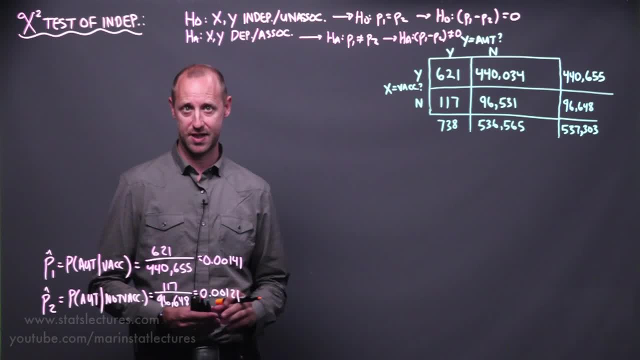 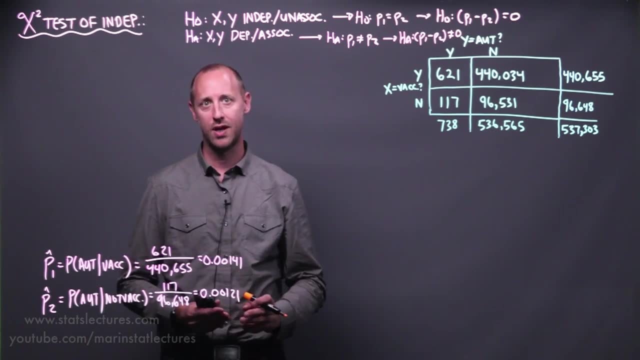 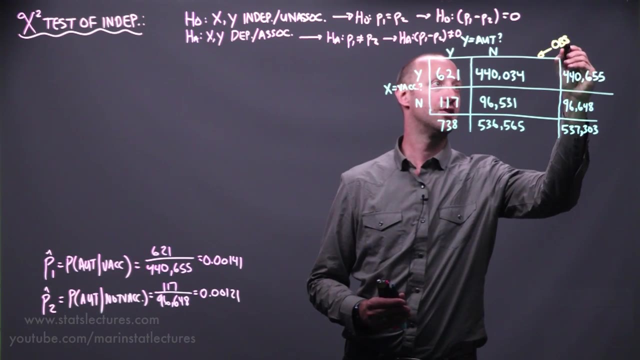 hypothesis testing. we're generally comparing what we observed in a sample to what we would have expected to observe if our null hypothesis was true. so, remember, we start by assuming the null is true and then see if we can provide evidence against that. so let's label that here. this, here is our. 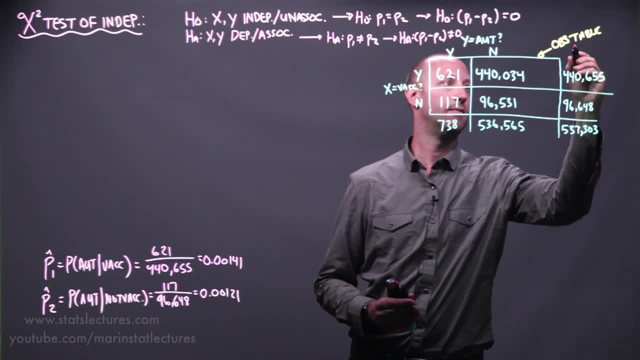 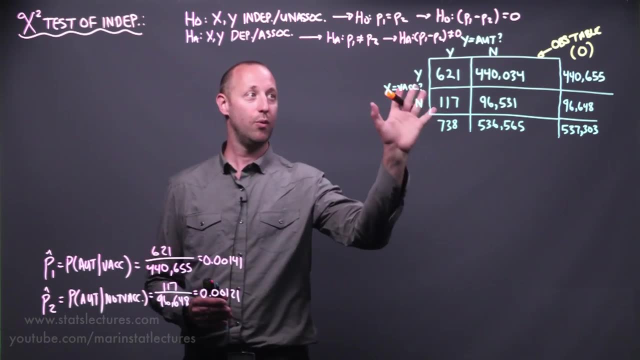 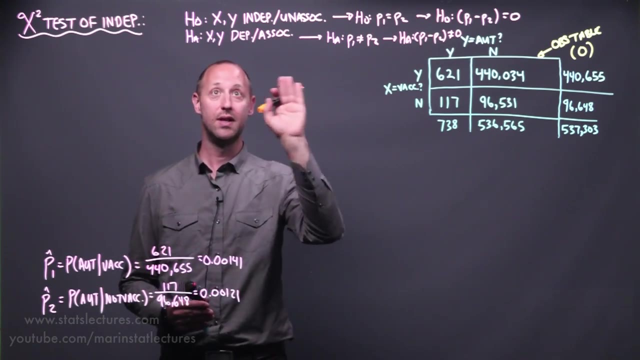 observed table which in notation, we're just going to use o to represent the observed values. so now what we'd like to work out is what we expect this table to look like if the null hypothesis really were true, if there are absolutely no association between X and Y or vaccination and autism. so here we have. 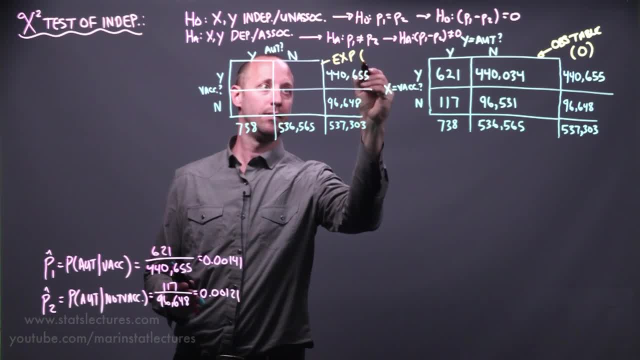 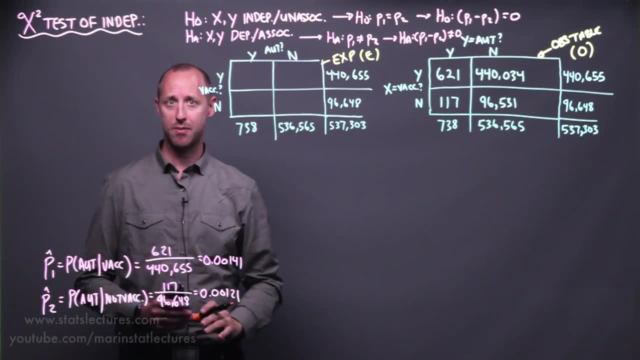 what we're going to label the expected table. yeah, with notation, we're going to use a capital E to represent this. So here we'd like to work out what we expect this table to look like if the null hypothesis really were true and there Was no association between x and y. 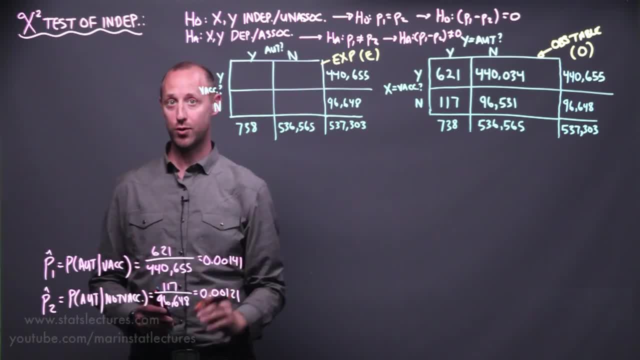 You'll notice, here We're going to keep the row totals and the column totals fixed. Okay, so the idea here is Thinking if we still had five hundred and thirty seven thousand three hundred and three people in our study- 738- who were diagnosed with autism. 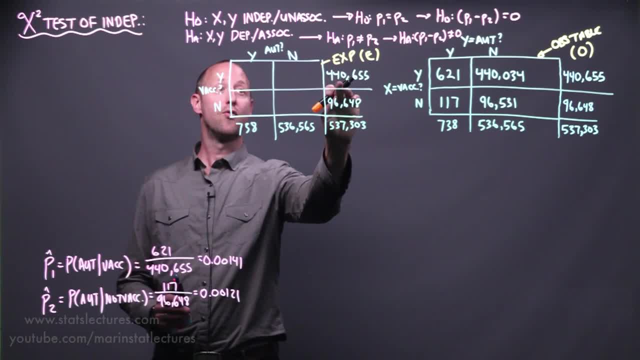 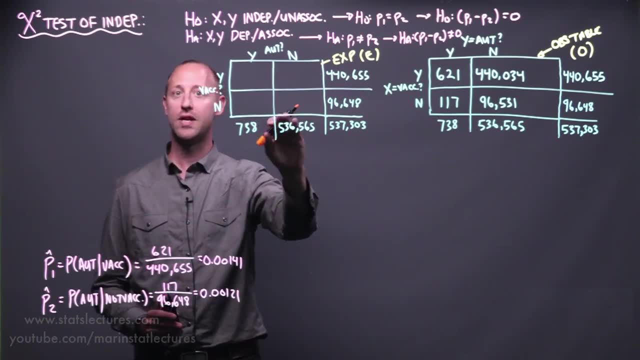 536, 565 who are not. if we still had 440, 655 who were vaccinated, 96, 648 who are not, how to expect people to be arranged inside the table? How many would expect to fall in each of these cells? So let's choose one of the cells to pick on, and I'm going to choose this cell up here. 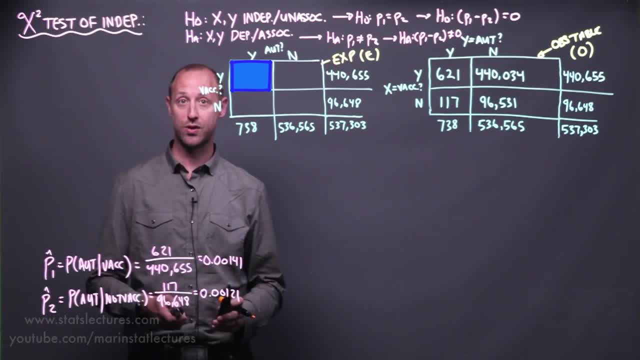 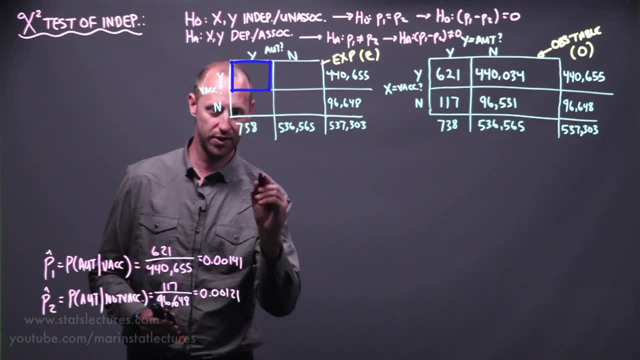 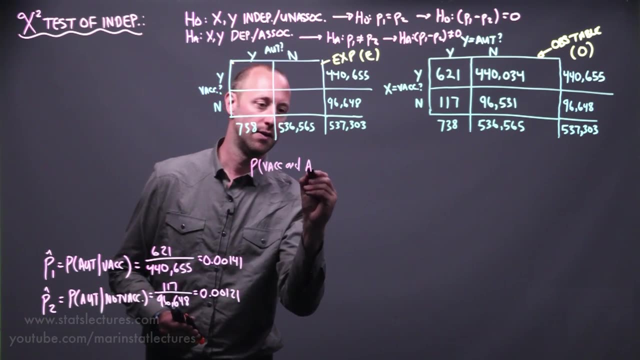 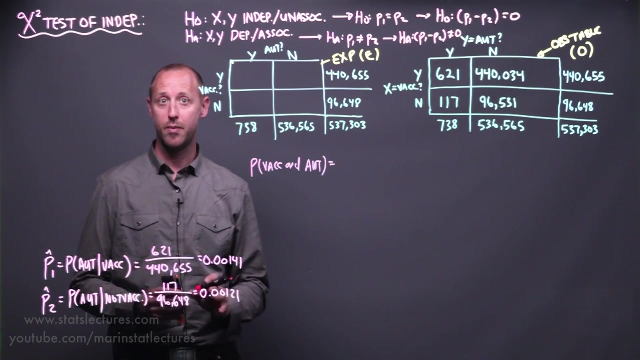 Those were vaccinated and those who also were diagnosed with autism. So what we'd like to work out is: What's the probability of falling in this cell? and we're going to start there- What's the probability of being vaccinated and Being diagnosed with autism? You know, you may recall, a rule of probability: the probability of a and B both occurring is 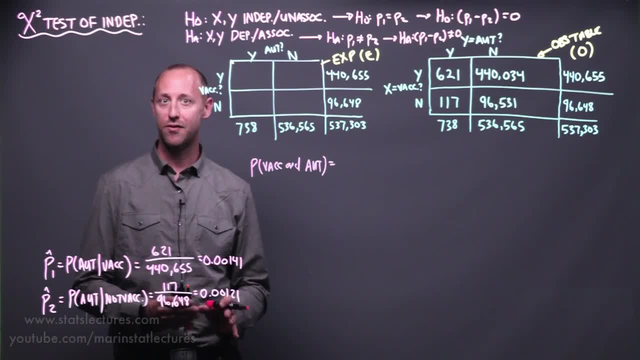 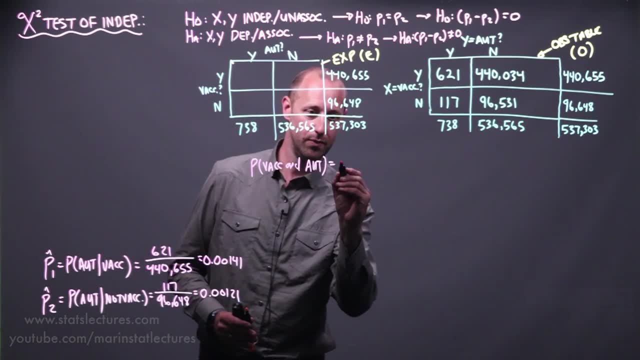 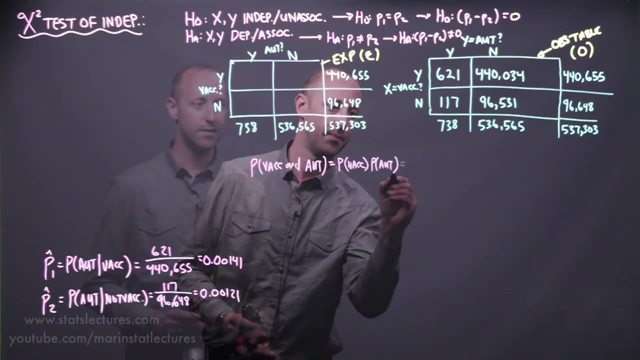 The probability of a times the probability of B. if a and B are independent, right here in our null hypothesis, We're assuming vaccination autism are independent, So we can express this as the probability of being vaccinated times the probability of development Autism now in our sample. Okay, the probability of being vaccinated. 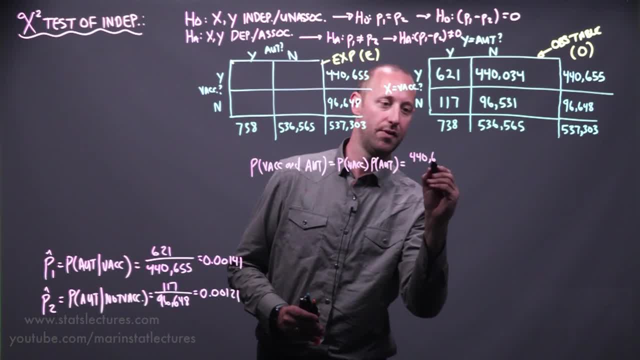 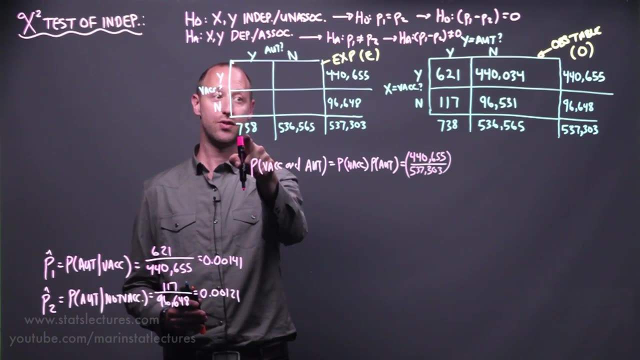 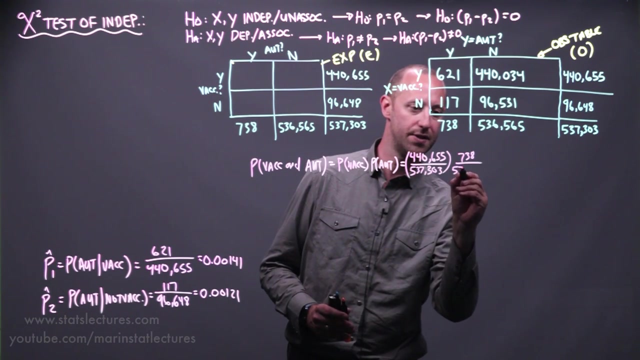 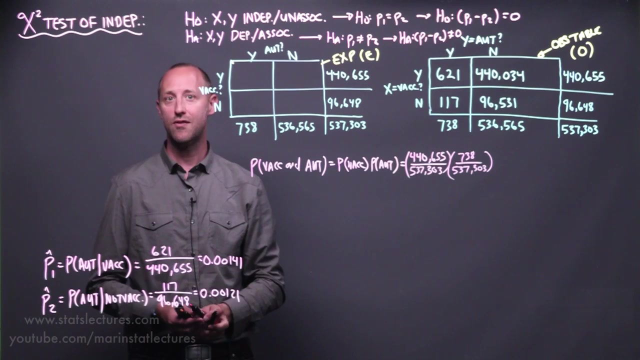 440 655 were vaccinated out of the 537 303. So this is the probability of being vaccinated and the probability of being diagnosed with autism. 738 out of the total were so 738 out of the 537 303. So this here tells us the probability of falling into that cell. if X and Y, if vaccination, autism, are independent. 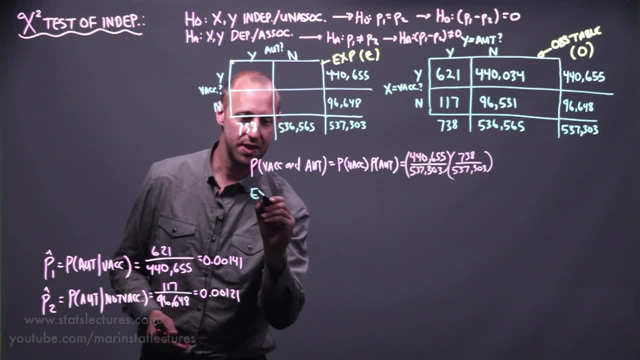 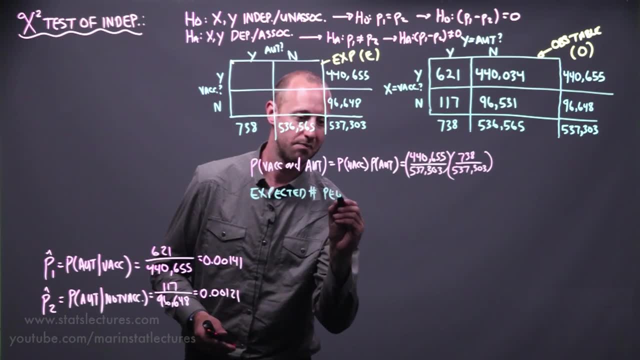 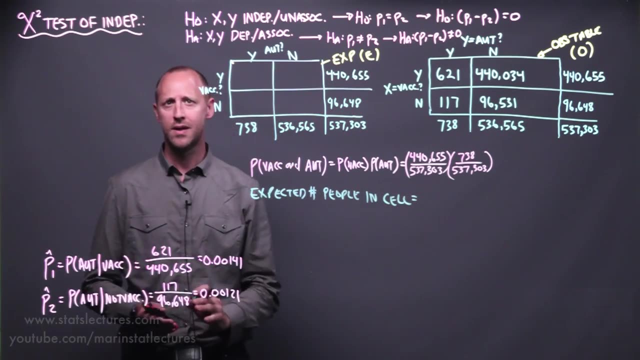 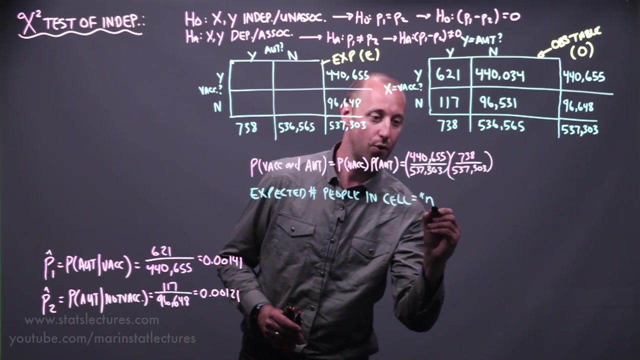 What we'd actually like to get at is What's the expected Number of people In the cell? now, you may recall from earlier stuff You've learned that to find expected number We're going to look at The total number of people in our study times. the probability of falling in that cell care n times P. 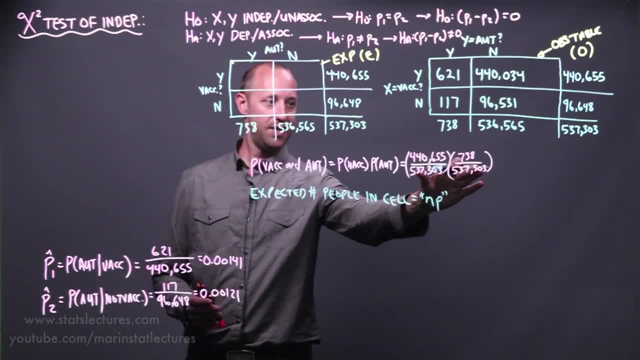 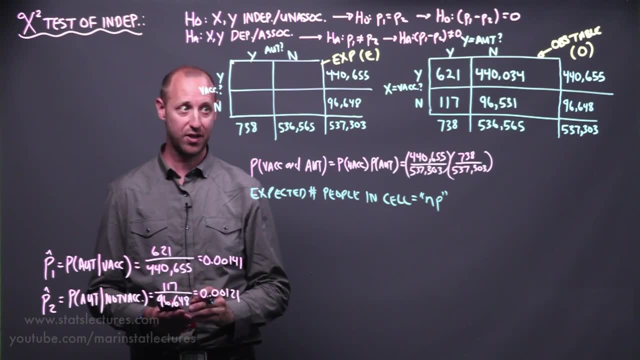 And so again, we can think of this here- Tells us what's the probability of an individual falling in that cell, and if we want to know how many we would be Expect to fall in that cell, we're going to multiply it by the total number of people. 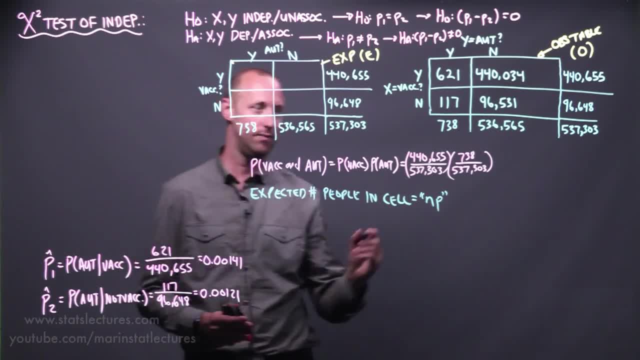 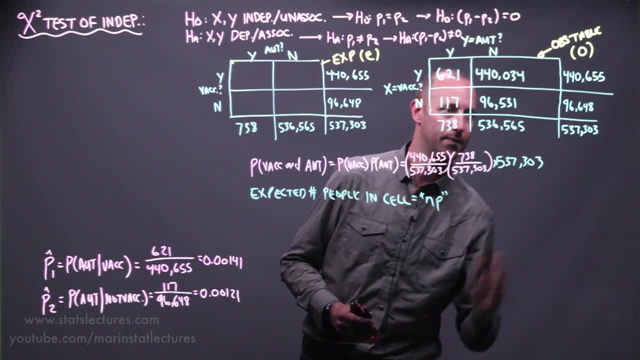 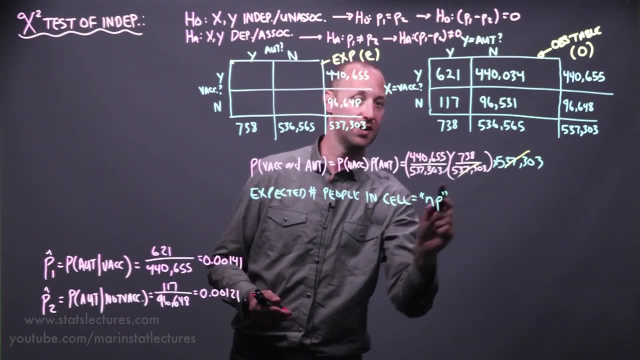 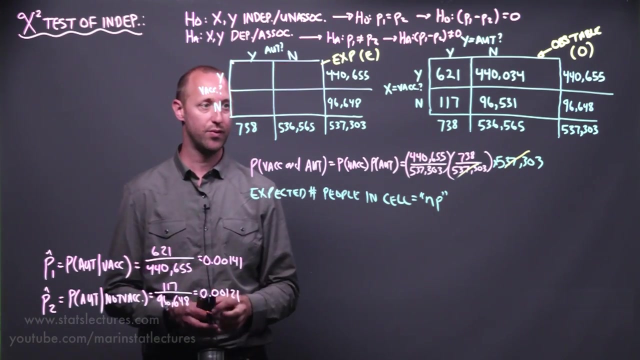 The total number of people times the probability of falling in that cell. so multiply it by the 537 303. Now one thing you may notice is that here One of these are going to cancel out, we're left with 440 655 times 738 over 537 303. 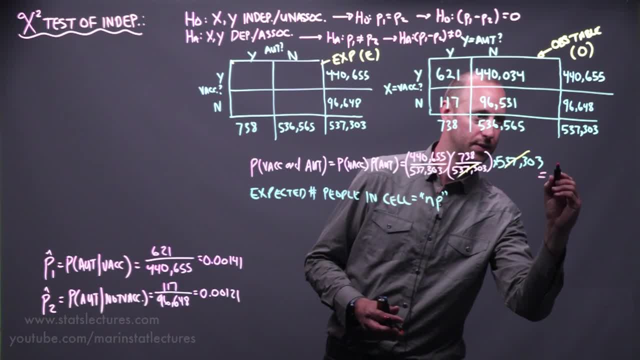 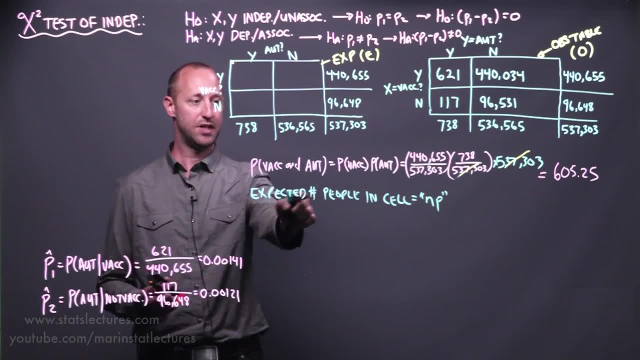 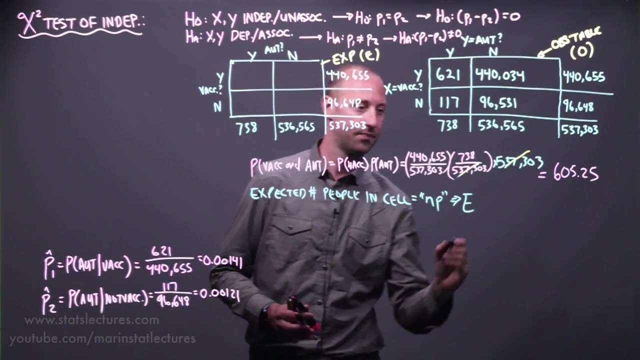 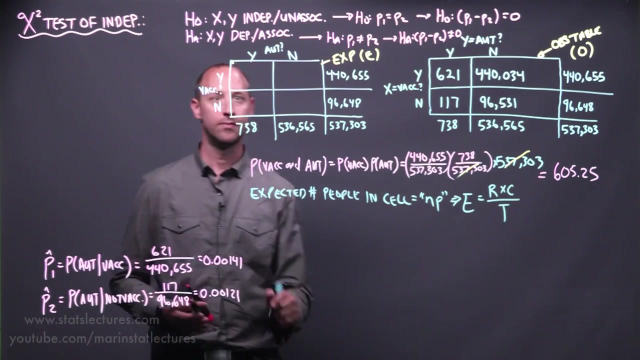 Numerically that's going to come out to be 605 point two five, And worth noting here the expected number of people falling into each of these cells. Sometimes written as capital E is The row total times the column total divided by the overall total. So if we want to know how many people do we expect to fall into this cell here, 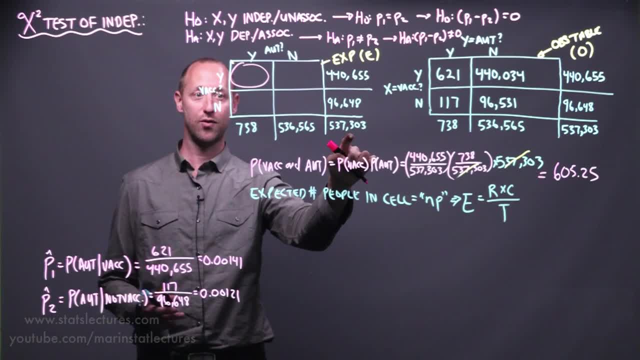 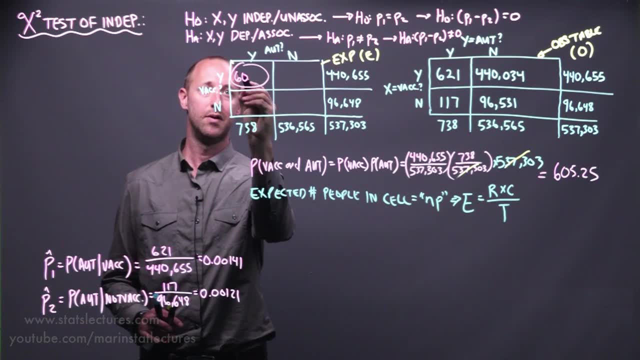 It's the row total times the column total divided by the overall Total. it's so often when you see this stuff presented in textbooks, they give you this formula for the expected cell count. What we want to do here is get some intuition as to why is this the formula for the expected cell count? 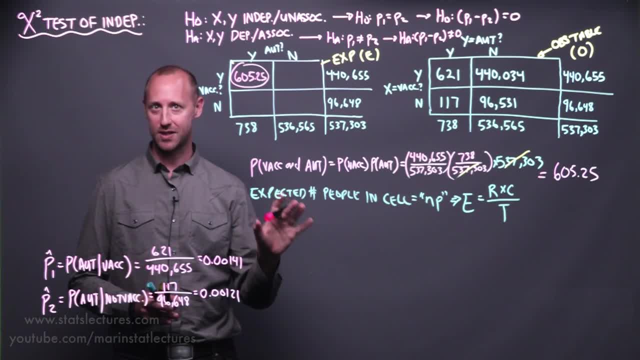 So remember we're not going to focus on plugging into formulas and calculating values. That's not an important skill for us to build, but it is important for us to understand the underlying concepts and calculations that are going into these. when we use a piece of software to 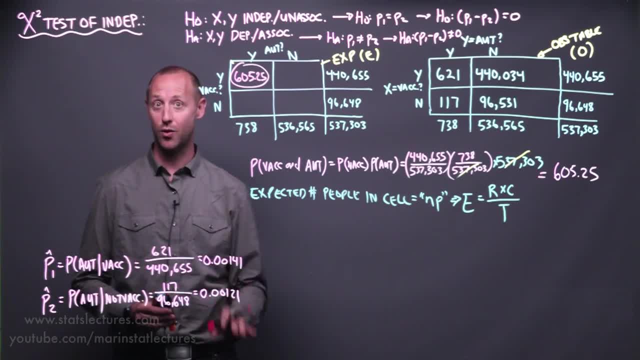 Get ourselves to the end values. One other important thing to note now is bring ourselves back to this idea of degrees of freedom that we've touched on throughout throughout these series of videos. So we can notice, with this table We've started with four cells, or we can think of as having four pieces of information. 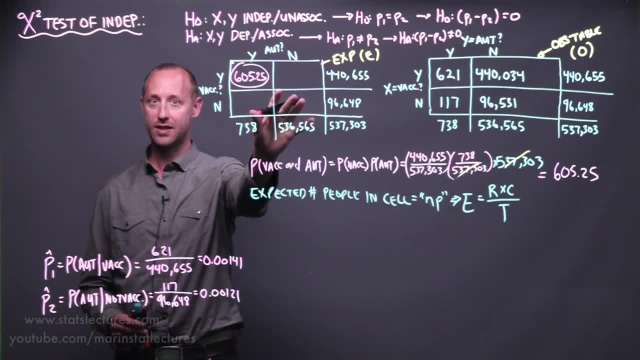 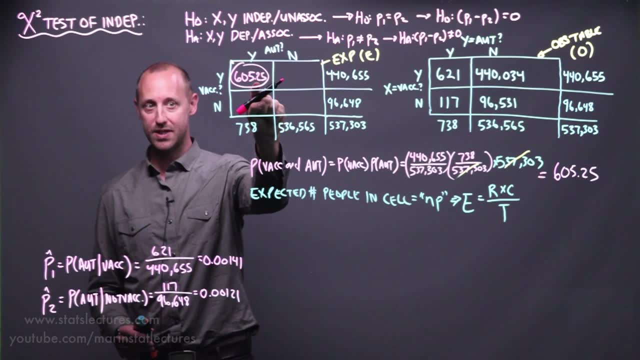 How many people fall into each of these cells. but taking a look at this, here the expected table We've started to build. Hopefully you can notice, we actually only have one degree of freedom Once this has taken on a value. This here, the value in this cell is going to have to be a fixed number in order to get back. 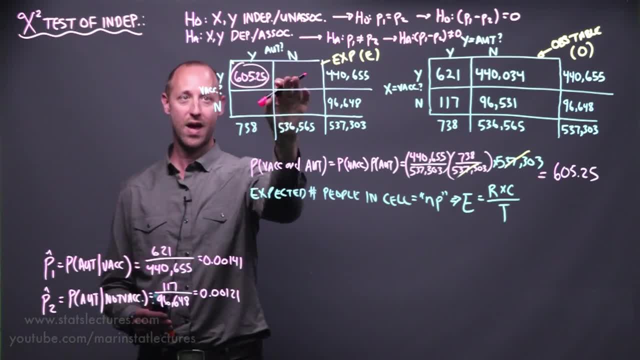 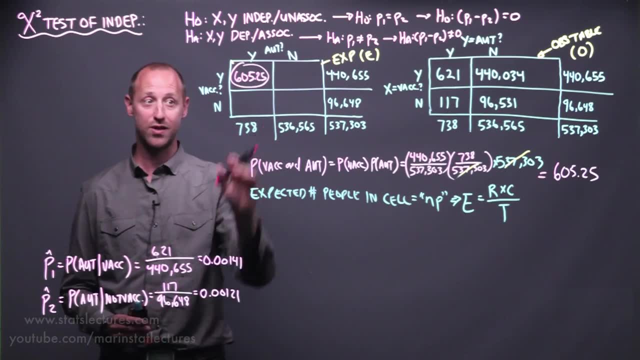 To that column total of 738, and so we have kind of four piece of information. We actually only have one degree of freedom And so let's go in and fill in the rest of the values for the expected table here. So we're notice this has to be. 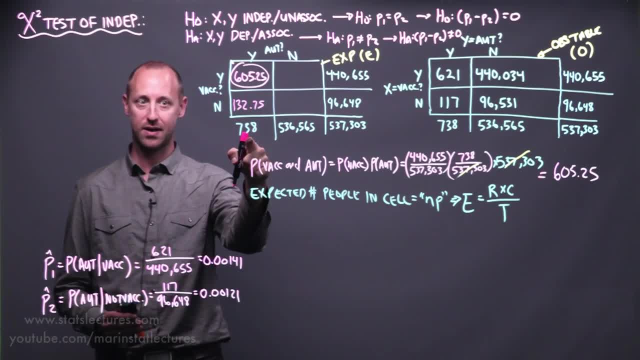 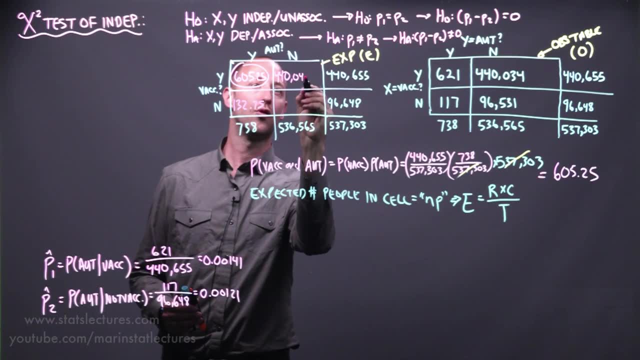 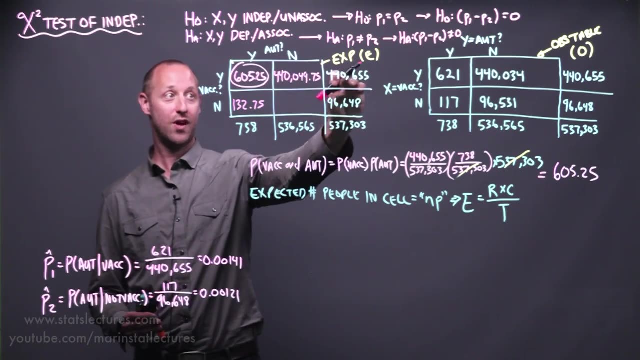 132.75. and again, to get us back to that column total of 738, this here: 440 049, 0.75. Okay, and again. you can get to these values by either Figuring out which value gets you back to that row total or by plugging this formula here: 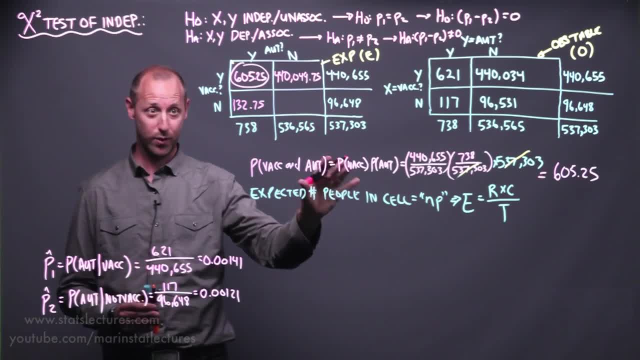 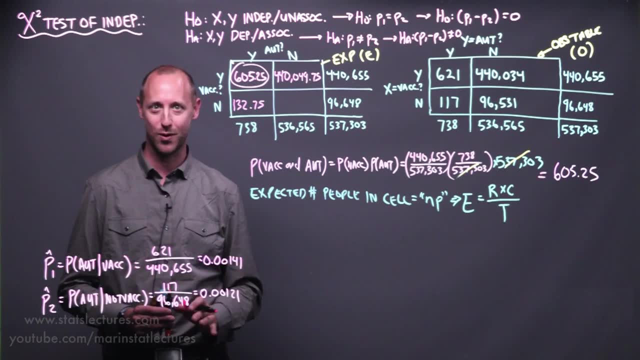 But again, as noted, we're generally going to do this stuff using software. It's going to get us right to the end. We just want to understand what calculations is a piece of software doing. So we're not using a kind of black box approach where we throw some data into a computer and it spits out some numbers. 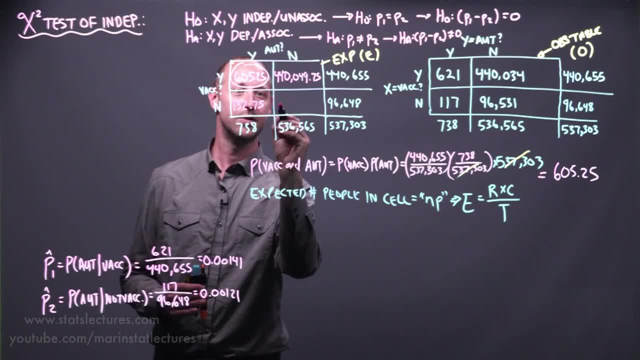 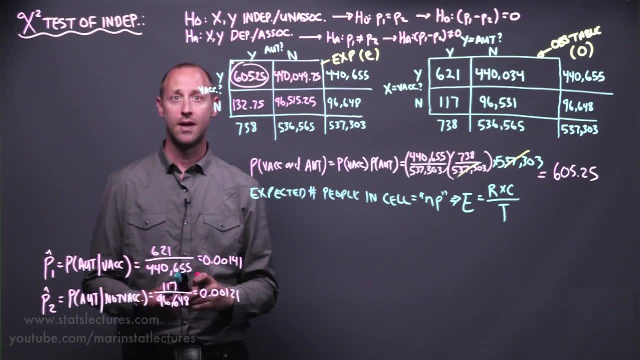 We want to know. how did it get those for us? So this final value: 96 515, 0.25. now I want to bring you back to a reminder: Hypothesis testing. we generally want to compare. what do we observe in a sample? 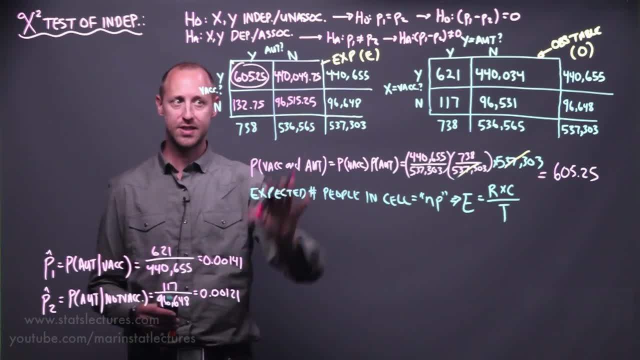 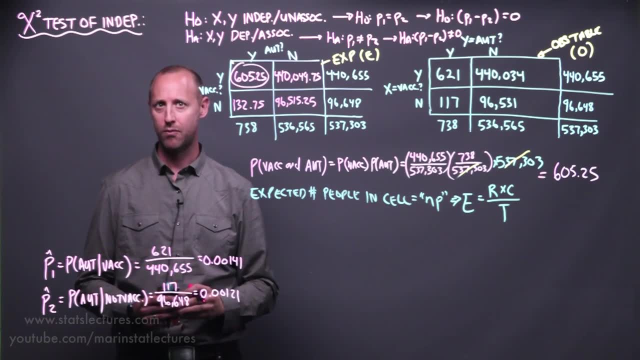 To what we've expected to observe if the null is true in some way right. When we did the one sample t-test, it compared our sample mean to the hypothesized value for the mean. When we did a difference in means test, we compared the sample difference in means. 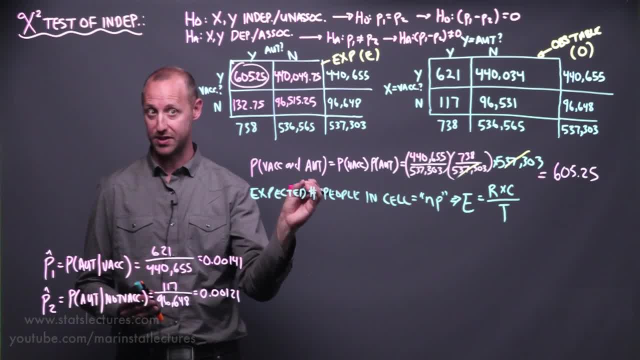 How far is that from what we'd expect if the null is true? right, zero or no difference. So we want to get it something that gets us the same idea of comparing what We observed to what we'd expect to have seen if the null is true. 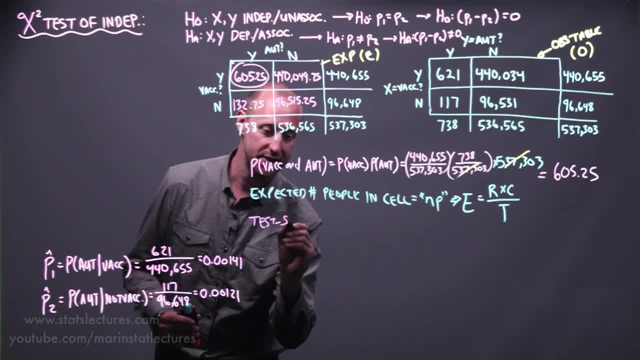 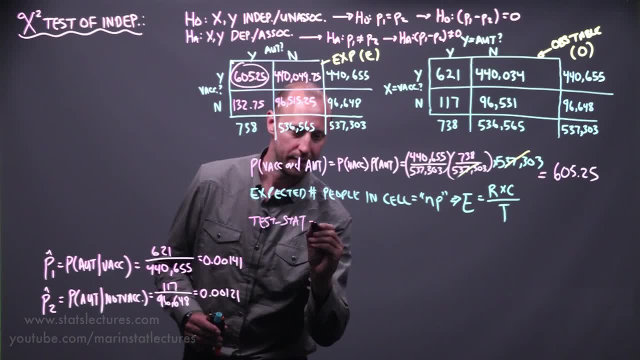 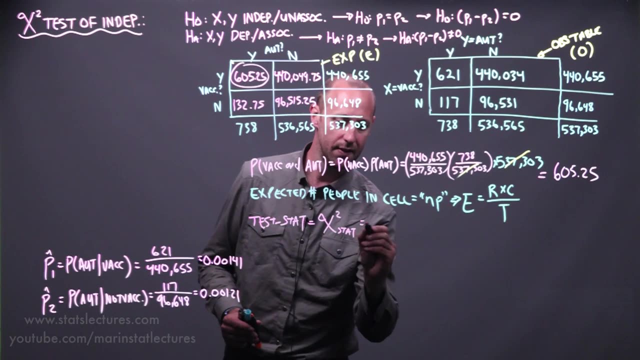 In order to do that, we calculate what we call a test statistic. All right, so these test statistics generally in some way compare observed to expected, And here we're going to call it a chi-squared statistic. To get this, we're going to sum over all the cells in the table. 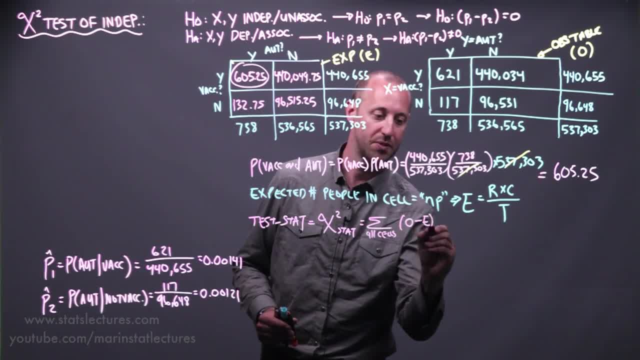 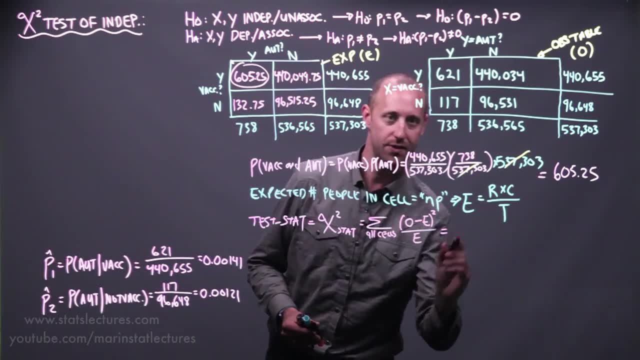 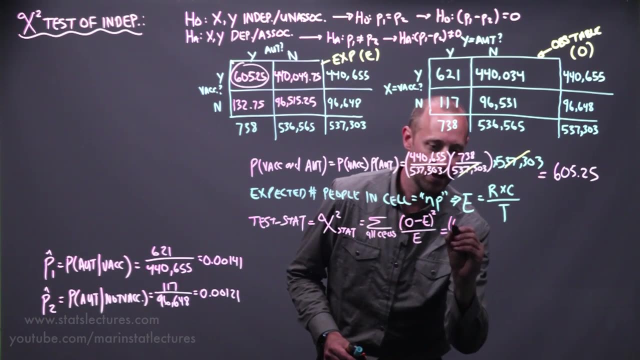 How far is the observed from what would be expected squared divided by the expected? And so let's go through and sub in some of these values again, just to see how we get ourselves to this test statistic. Let's start with the first cell here. our observed cell count was 621. 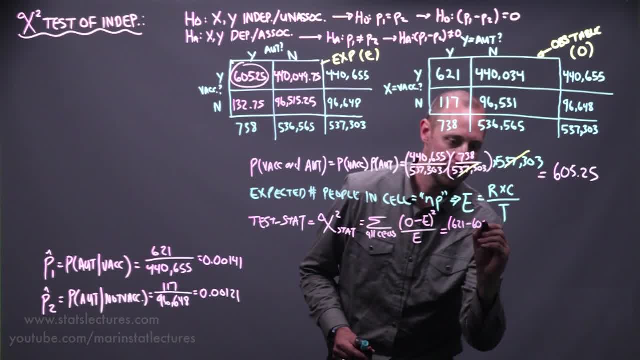 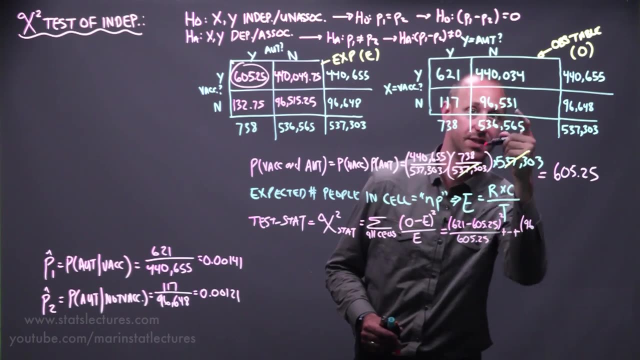 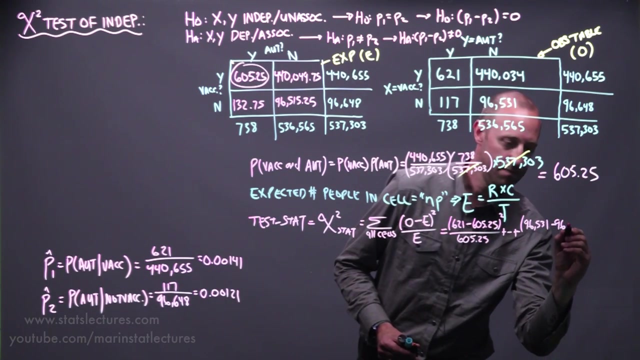 and how far is that from the expected of 605.25? we square that divided by the expected cell count of 605.25. so I'll just jump to the last one here. how far is the observed ninety six, five, thirty one from the expected count of ninety six, five one, five point two, five. 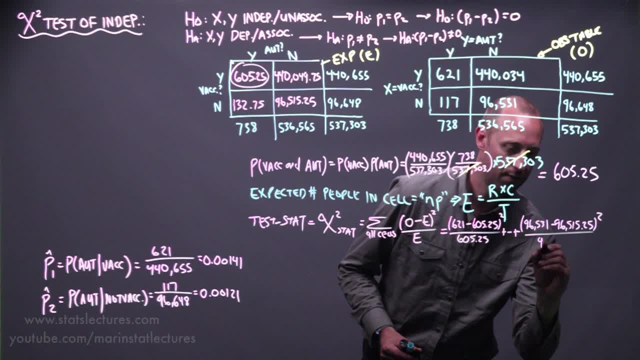 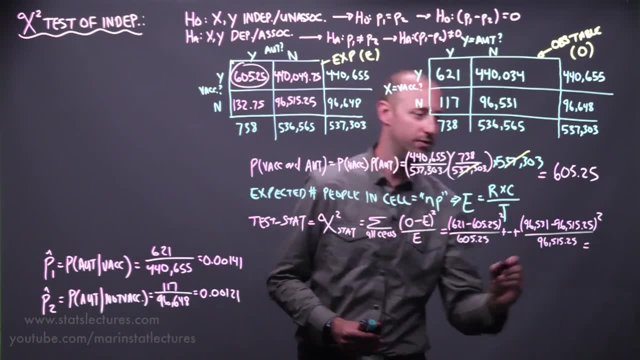 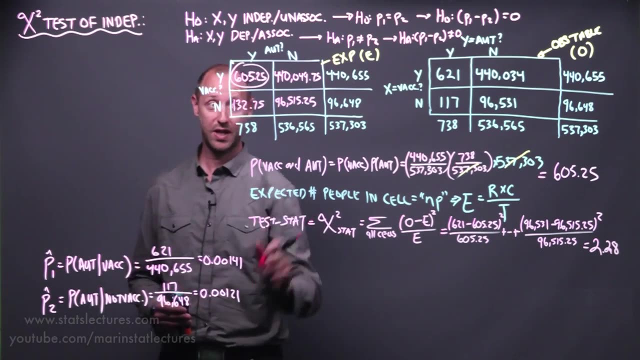 squared divided by the expected count of ninety six, five, one, five point two, five and if you work all this out it's going to come out to be two point two, eight. this test statistic follows some distribution. it follows a chi-squared distribution similar to what we've seen earlier. right the t-test, we assumed our. 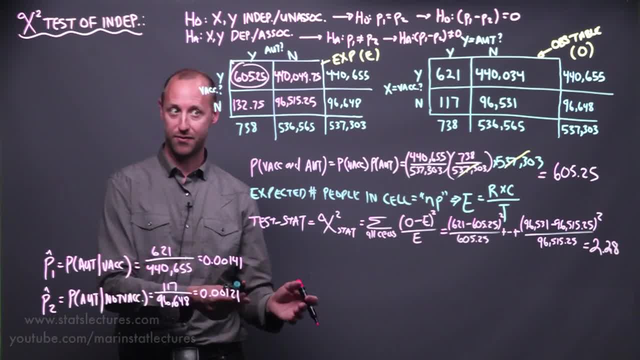 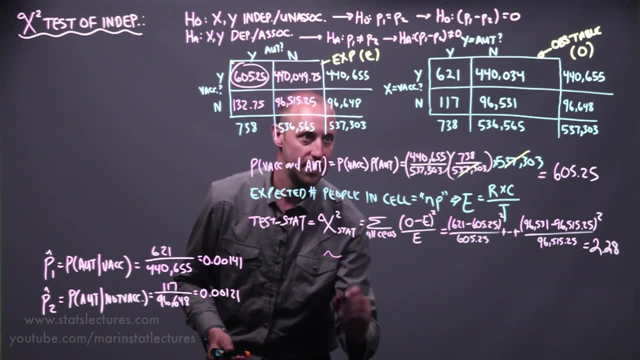 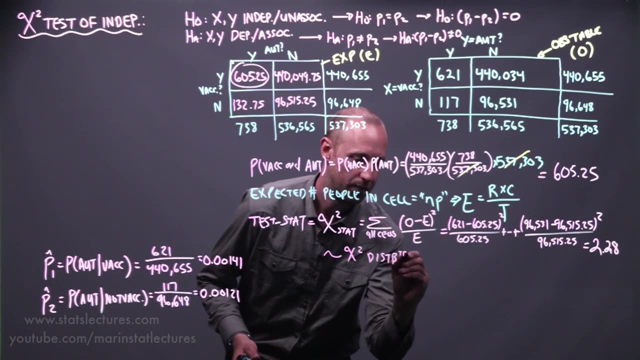 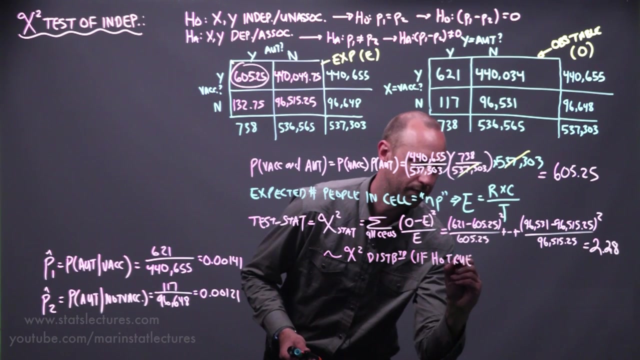 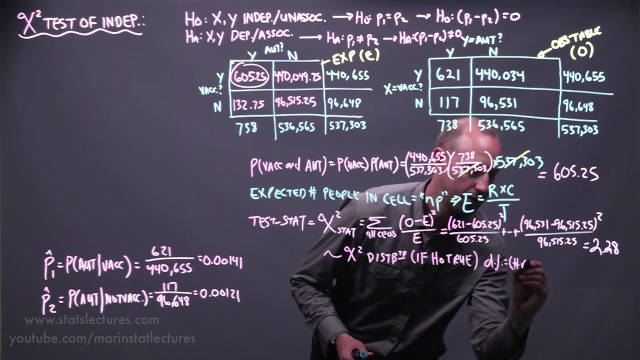 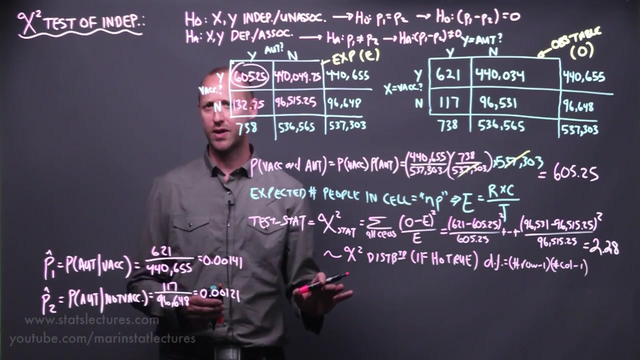 test statistic followed a t distribution. ANOVA. it followed an F distribution. so here's another theoretical probability distribution. this test statistic is approximately chi-squared distributed and if the null hypothesis is true and it has degrees of freedom, the number of rows minus one times the number of columns minus one. and again we don't. 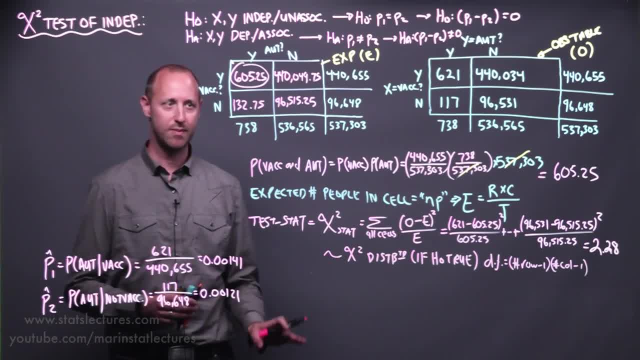 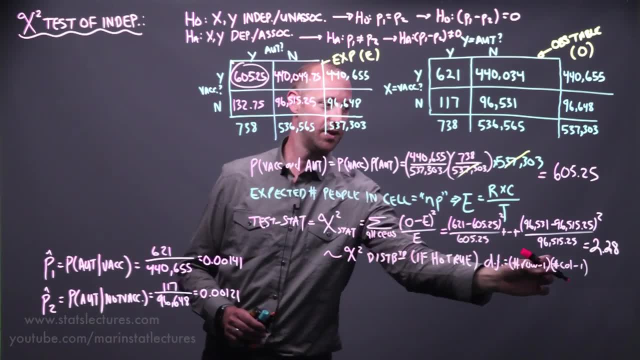 want to get stuck on formulas calculating degrees of freedom and so on, but I want to bring you back to what we talked about earlier. right, two rows, rows, two columns. 2 minus 1 times 2 minus 1 is 1, right, that: one degree of freedom. 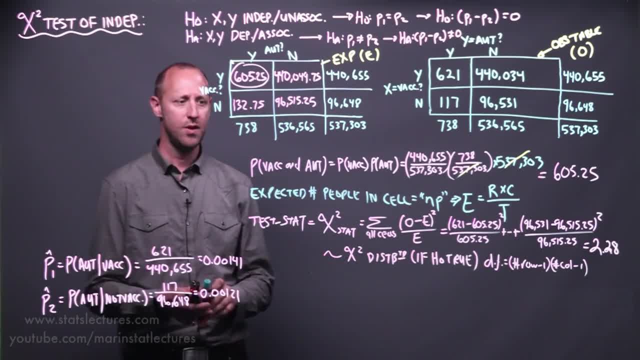 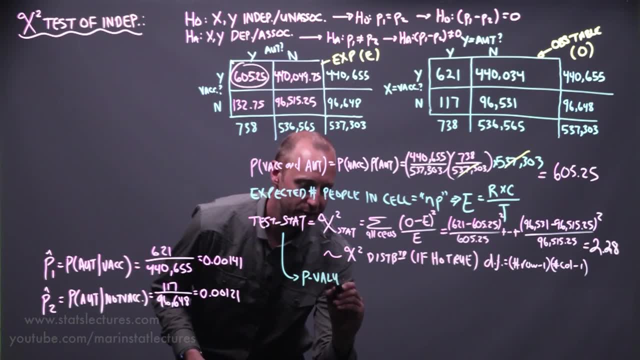 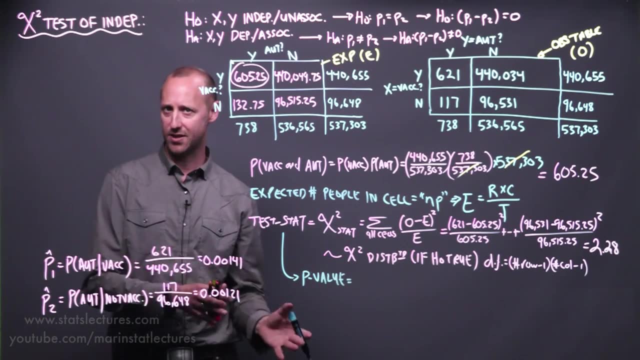 that we talked about a little bit earlier. Okay, and then, like always, we convert our test statistics into p-values and p-values, while the way of getting at the exact numeric value changes slightly depending on if we're doing chi-square tests. analysis of variance. 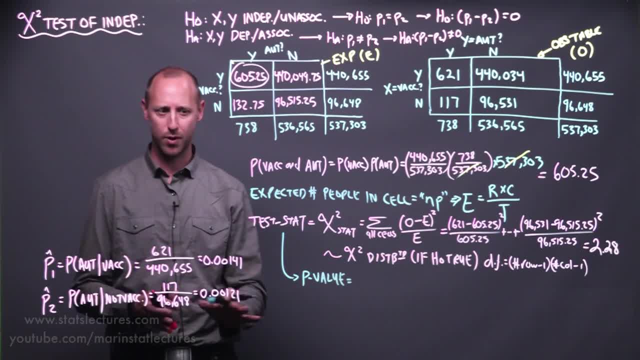 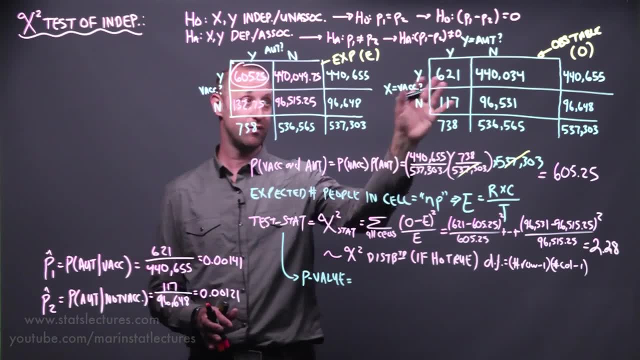 if we're doing parametric or non-parametric or bootstrapping type approach, the mechanics change a bit. the underlying concept is always the same. We're always trying to get at what's the probability of observing what we did in our data or something even more extreme. 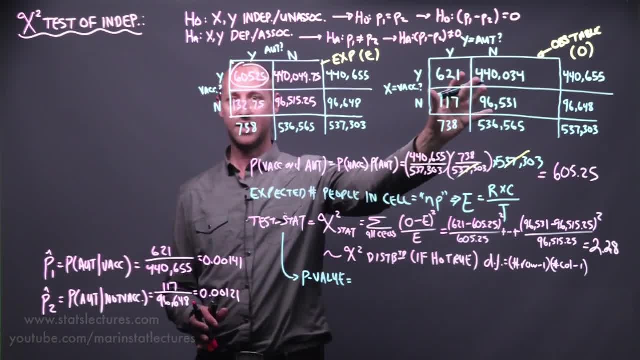 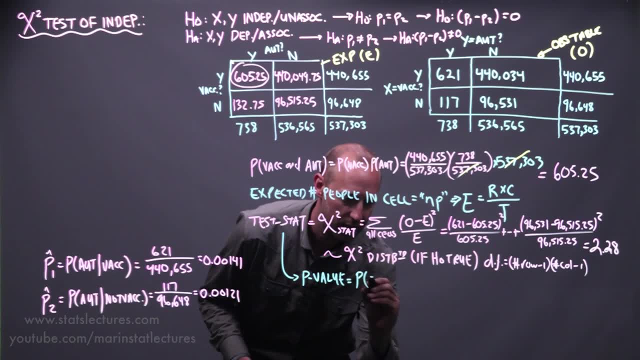 if our null is true? What's the probability of seeing a table that looks like this if the null is true, and we'd expect it should look something like this, Or what's the probability of getting a chi-squared statistic greater or equal to what we observed if the null? 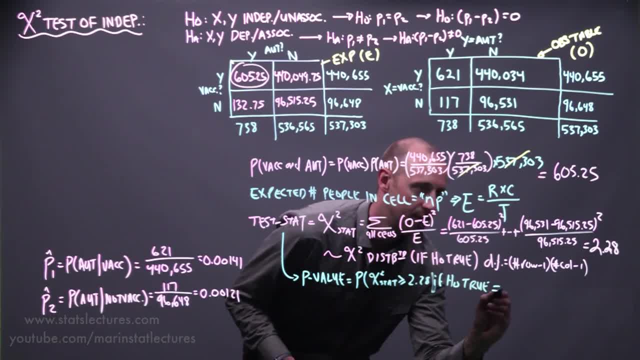 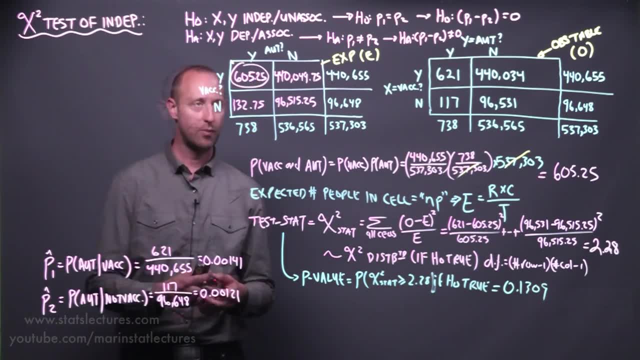 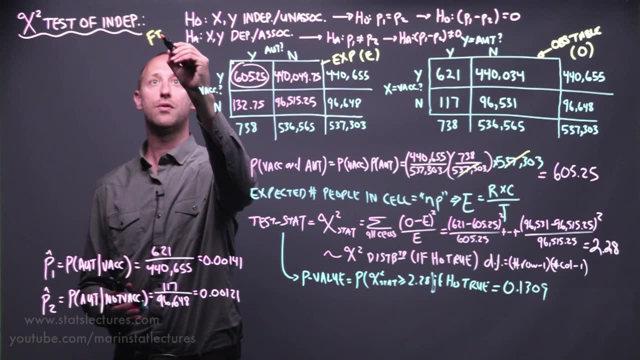 hypothesis is true, This is going to come out to be 0.1309,. okay, or about 13.1%. With that, what are we going to do? Our p-value is bigger than an alpha of 5%. we're going to fail to reject our null. 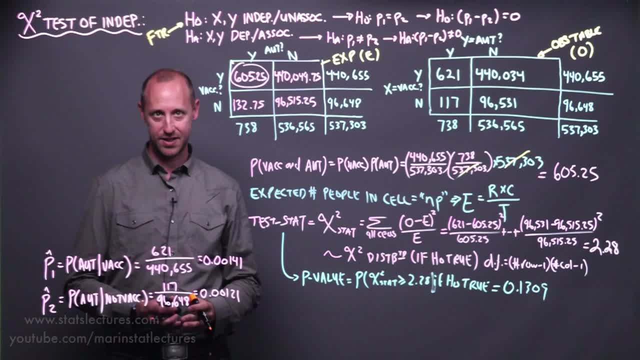 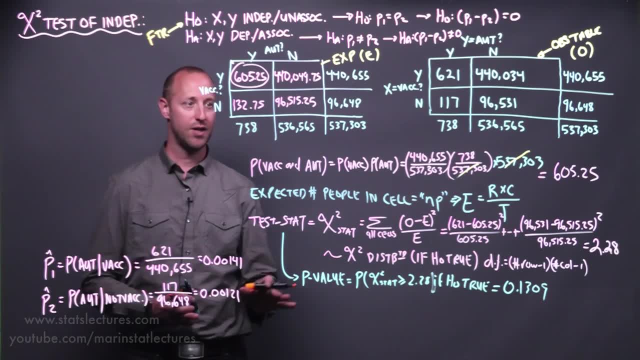 hypothesis right. our conclusion is: we do not have evidence to believe that there's an association between vaccination for MMR and development of autism. I also want to bring you back to a reminder about test statistics. The larger they grow, the larger they are in value. generally, the more evidence we have. 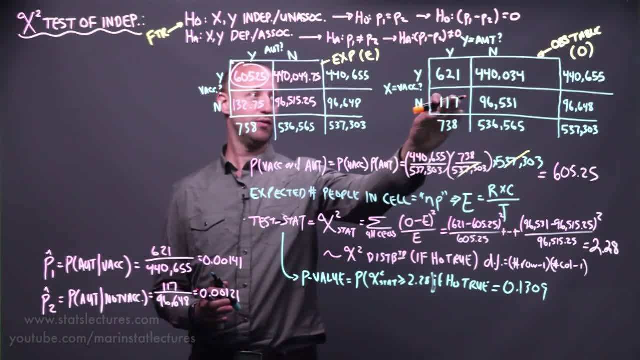 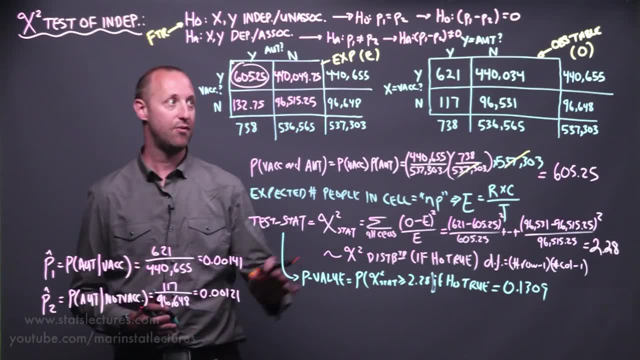 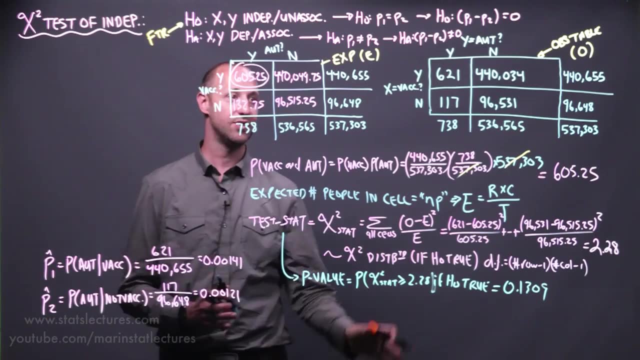 against the null. You can think here: if what we observed and what we'd expect were very different, our test statistic is going to come out to be a fairly large number. If what we observed and what we'd expect to see under the null are pretty similar, that tells us. 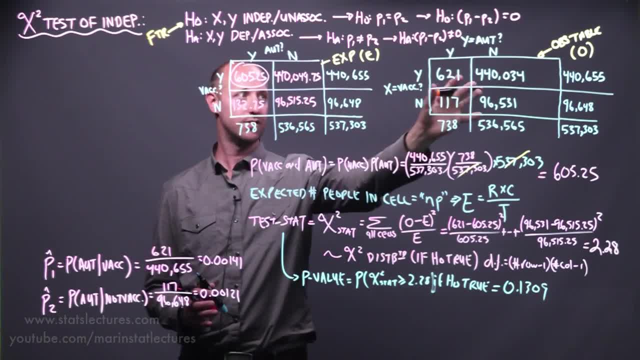 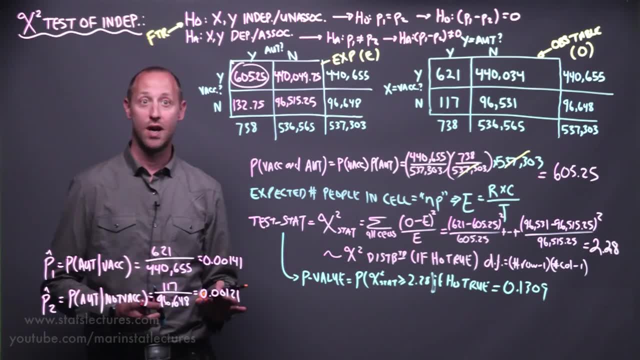 the null hypothesis is likely true, What we saw. what we saw and what we'd expect to see aren't very different. I also want to bring you back. I want to bring you back to some things we've talked about through these series of videos. 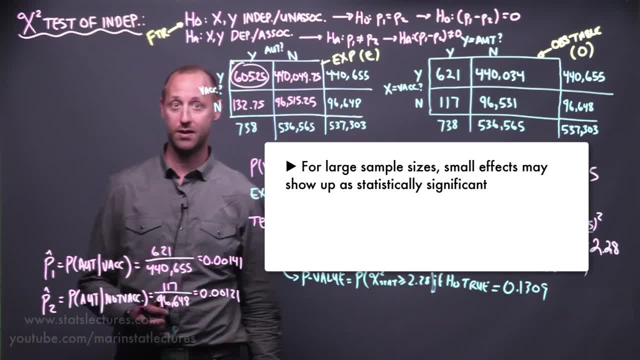 A reminder that for really big sample sizes- and we have one of those here for really large sample sizes- small differences sometimes can show up as being statistically significant. Also, for really small sample sizes, sometimes there may be big differences that don't show. 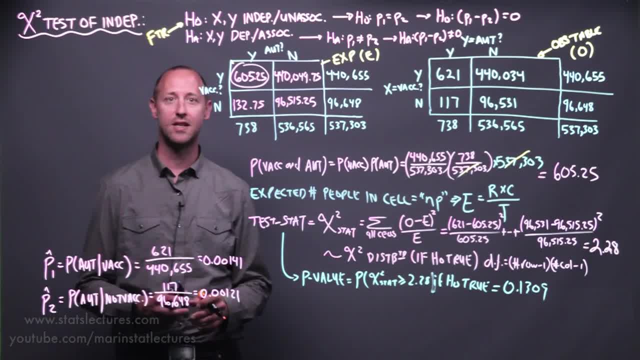 up as statistically significant. So I really want to bring you back to this idea that p-values are a guide. okay, they're a tool that we can use to help us make a decision. They're not a magic number. you know? greater than 5%, less than 5%? that answer our question. 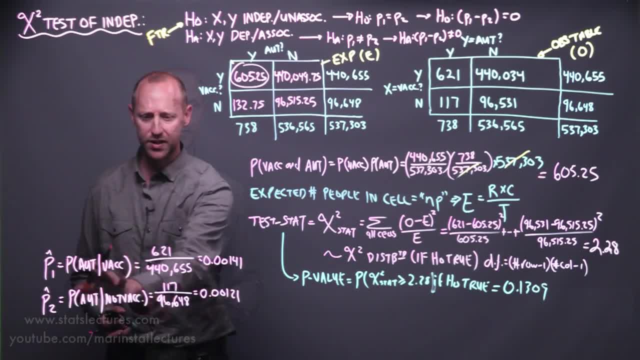 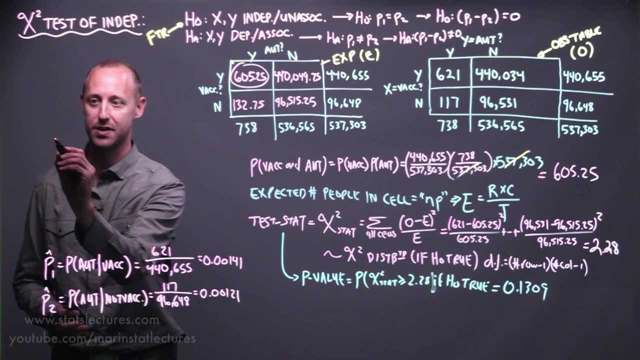 for us. you know, is vaccination harmful or not? We'll get to talking about these in a moment and how we can compare those, but first I just want to get to the idea of assumptions. Like all these large sample approaches, or even the non-parametric approaches, they all have some assumptions that are built into. 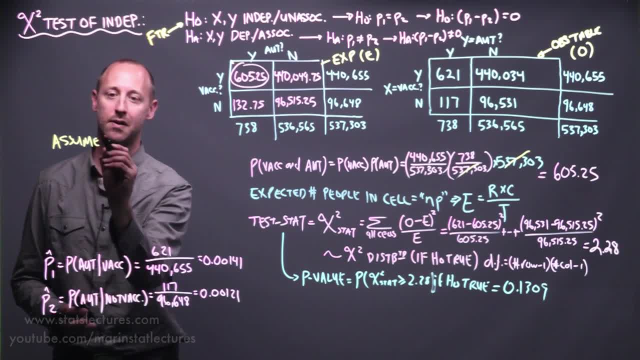 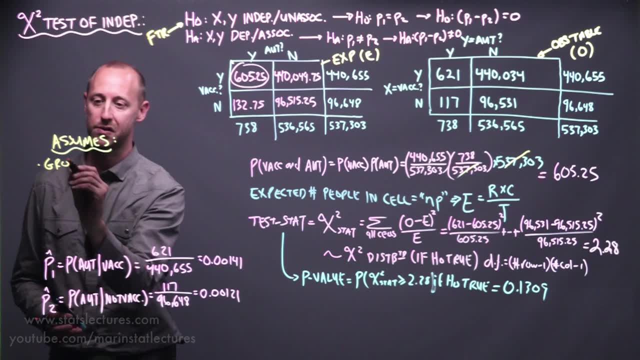 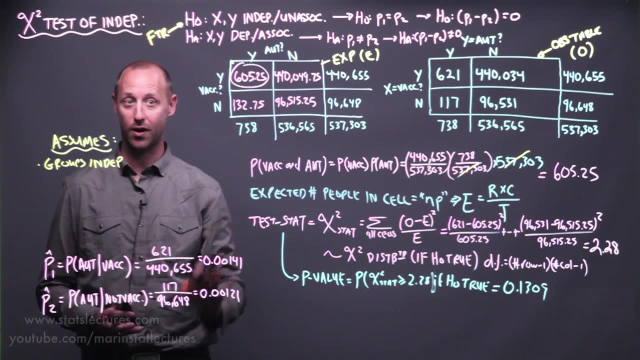 them. So, in order to work through the chi-square test, we're going to make a few assumptions. The first is that groups are independent, meaning that those who are vaccinated and those who are not are independent or different people. We're also going to assume that. observations: 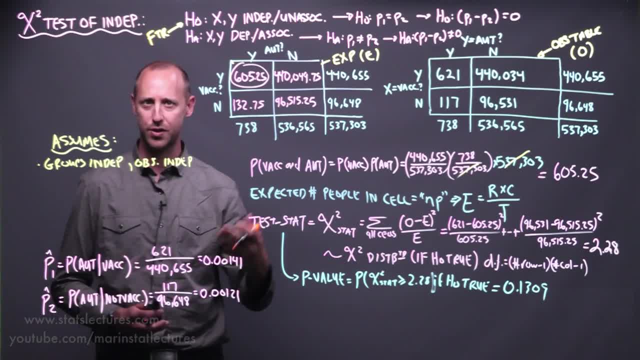 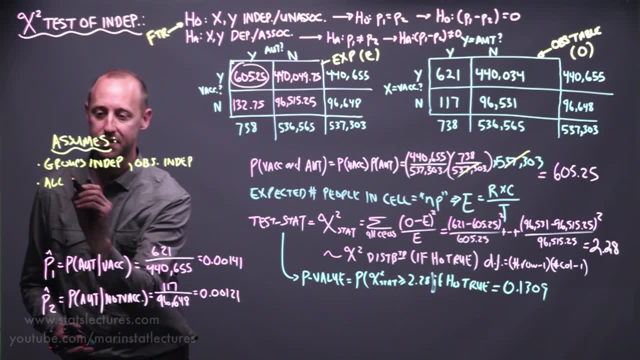 are independent. So person one, person, two, person, three, they're all independent of one another. Then, in order to do this test, we need all cells, all cell counts, to be greater or equal to one: 1.029667.0256.332. 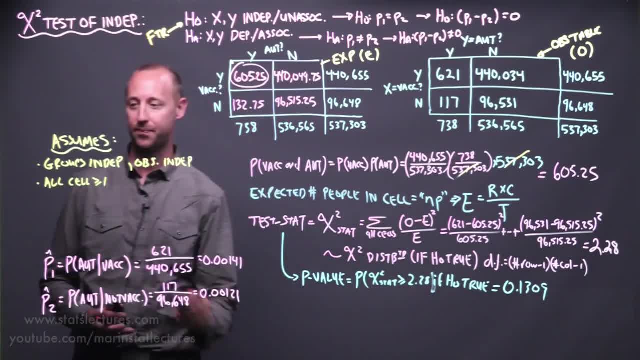 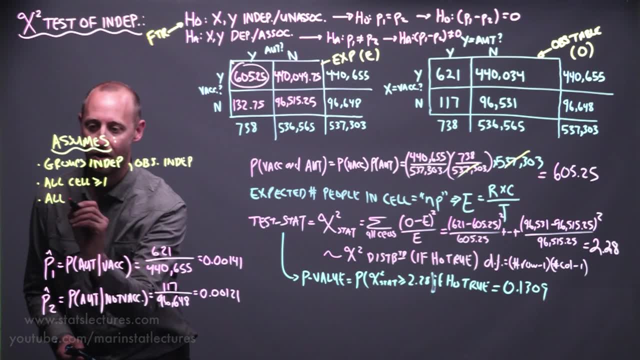 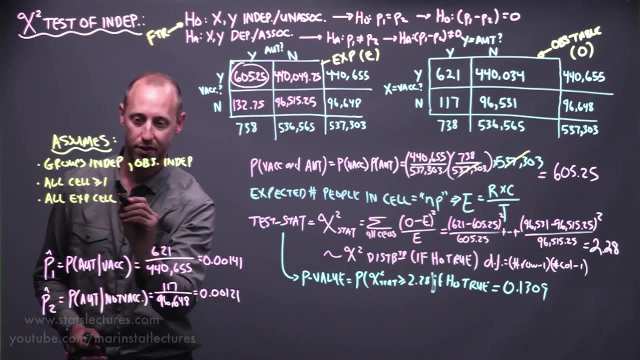 we need to have at least one person in each cell of the table and we're going to have a large sample requirement, like all these large sample tests do. and this is all of the expected cell counts, right, all of these here, the expected cell counts are greater or equal to five again, five being a. 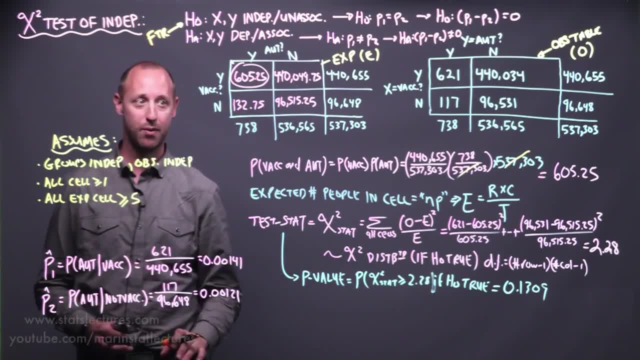 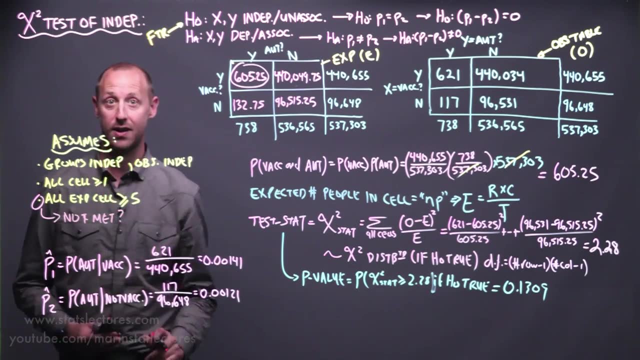 guideline. it's not a magic number. this is the large sample requirement that's necessary in order to do the chi-square test or in order to assume our test statistic follows a chi-square distribution. if this here is not met, if we don't have a large sample size or a large number of 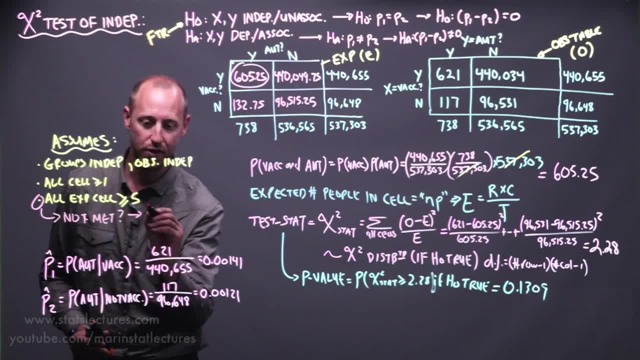 expected cell counts in each cell. some things we can do are use a nonparametric approach and carry use a I'm an exact test- this one's called Fisher's Fisher's exact test- or we can also try something like a bootstrap type approach. a few more just kind of technical details for us to mention. the first is that we 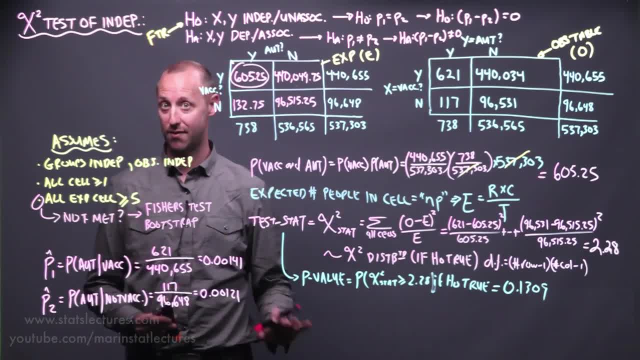 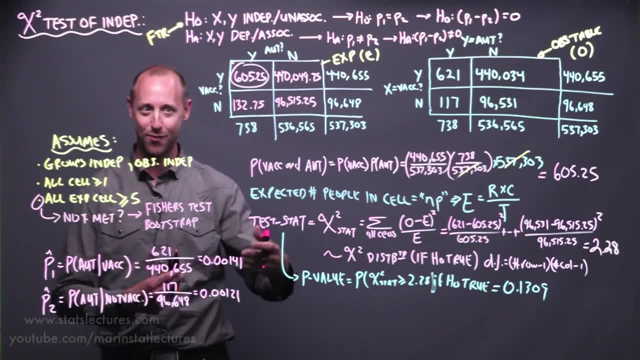 can do this chi-square test if the table has more than two levels for X or Y. so if we had you know, vaccinated, know a little bit a lot or some form like that, something had more than two levels, we can still do the chi-square test. it doesn't need only two levels. another note worth mentioning: 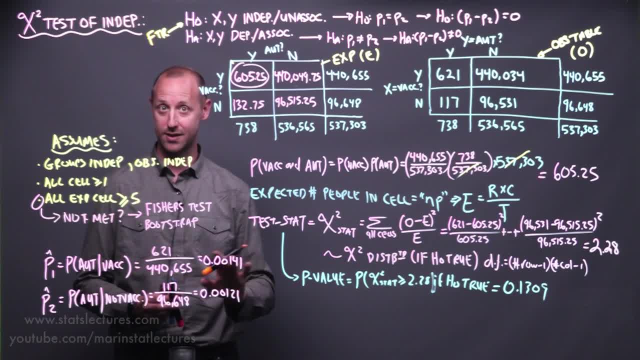 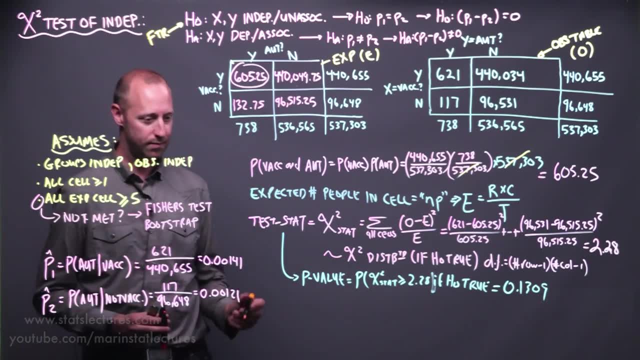 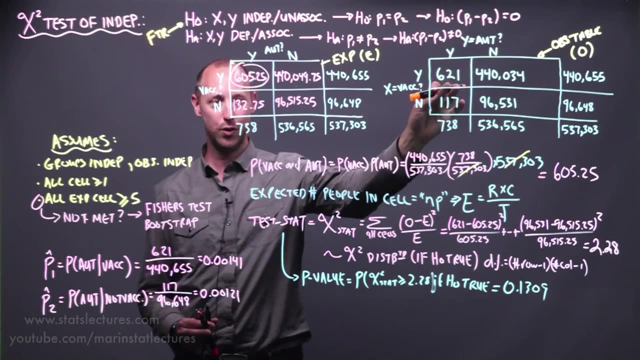 there's this idea of continuity correction. okay, it's called Yates continuity correction. I'll give a very quick kind of intuitive explanation of what that is. the idea is that here our accounts are on a discrete level, right, we have one person or two, or three or four in each. 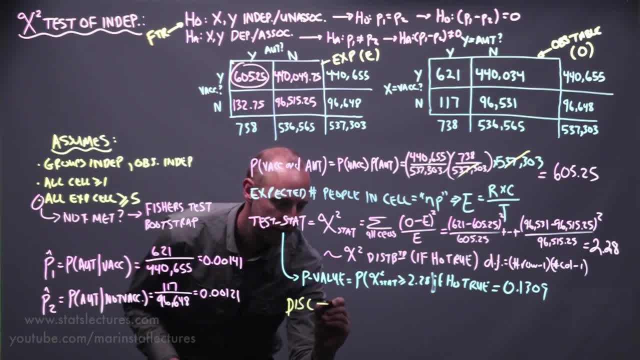 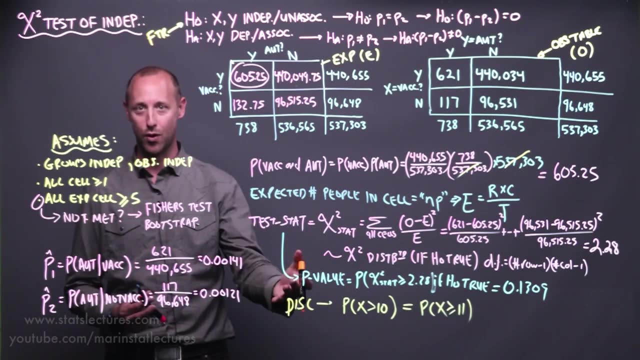 cell of the table. so on a discrete scale, the probability say that X is greater than 10. having more than 10 people in a particular cell is the same as saying X is greater or equal to 11.. more than 10, 11 or more mean the same thing when things only take on integer or whole values. 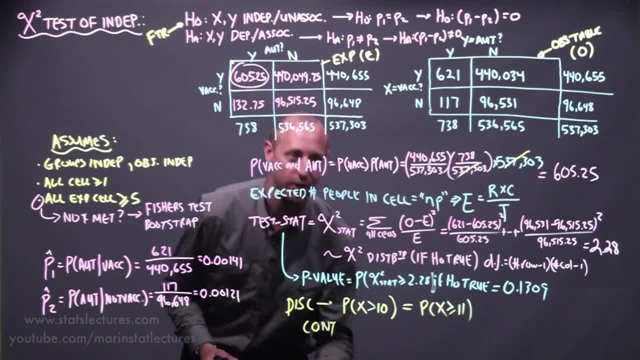 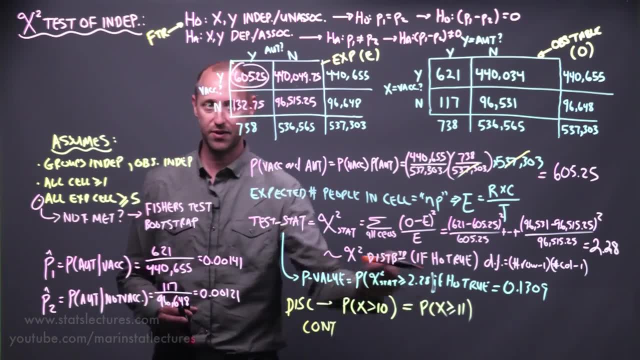 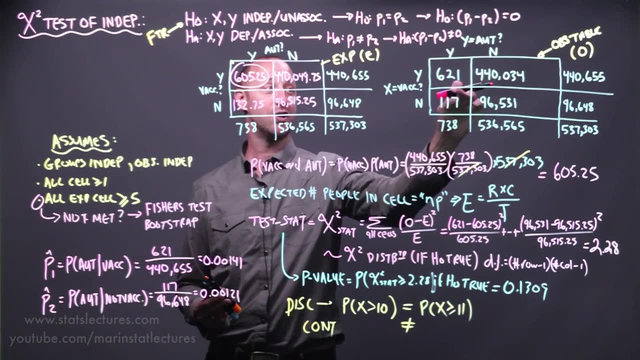 on a continuous scale. if we're looking something that's on a continuous scale and it can take on a value of 10 or 10.1 or 10.2 or so on, these mean different things. these are not equal. so that's the idea of the continuity. correction is that we're going from something that's measured. 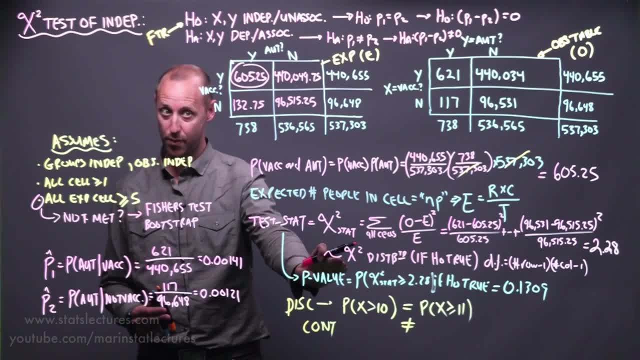 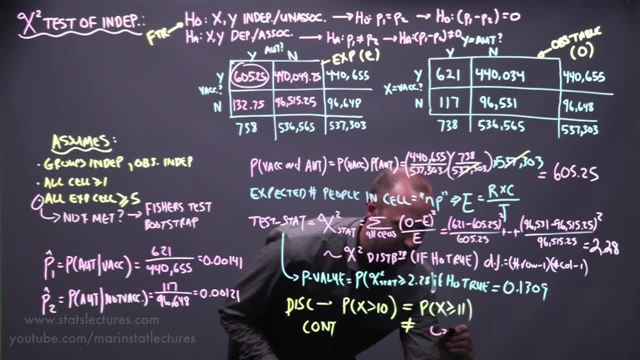 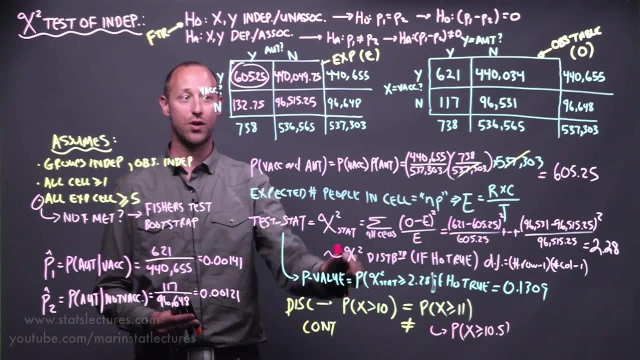 on a discrete scale and we're going to work out a p-value or probability using a continuous distribution and to correct for that. the kind of suggestion for this correction is to sort of split the difference and use X greater equal to 10.5, right, so take the two statements that are equivalent. 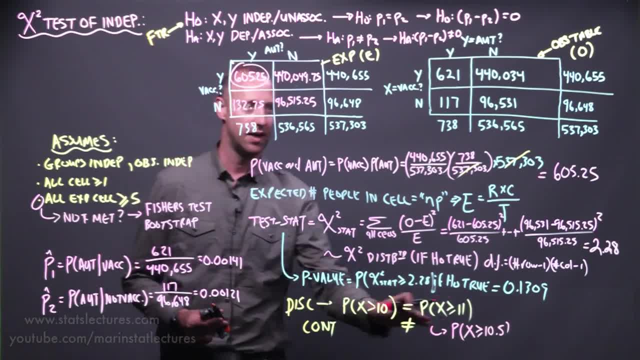 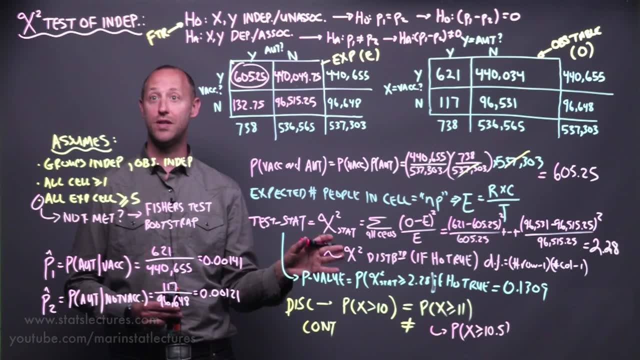 on a discrete scale, which are not equivalent on a continuous scale, and use the midpoint. now, one thing that we're going to get into following this is that the chi-squared test says nothing about the direction or the strength of an association. so if, okay, this is a really big if, because it's 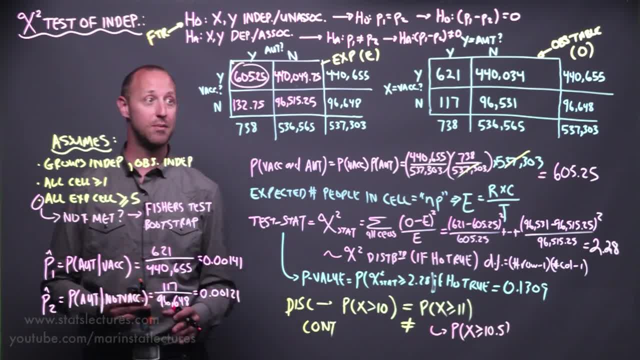 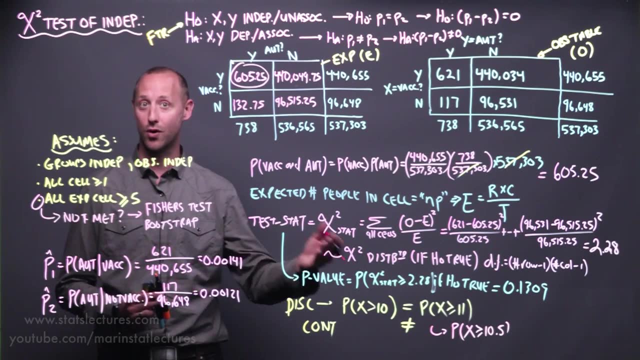 actually not true. but if we were to conclude that we have evidence to believe that vaccination for MMR and autism are associated, using the chi-square test, it wouldn't actually tell us: is vaccination making more likely or less likely to be diagnosed with autism? it also wouldn't tell us does how much more or how much. 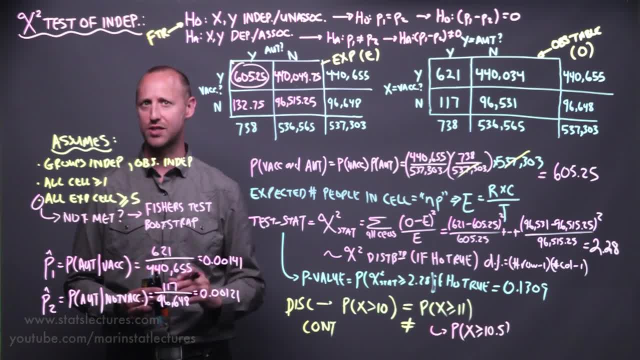 less likely. so you can kind of think of it as more like a screening test. it just helps us decide. do we think we have evidence that there's an association or is there not any evidence that there's an association? to look at measures, we can work with things like the risk difference or attributable risk, the risk ratio or the Oz. 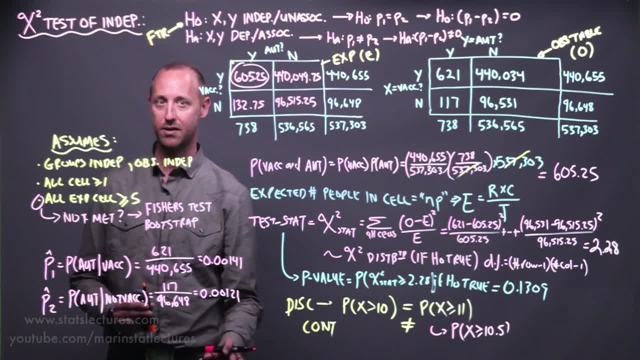 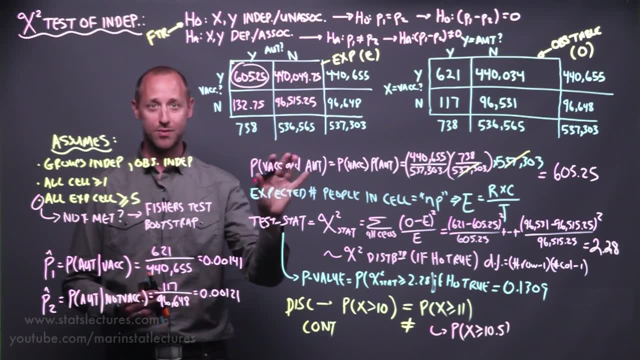 ratio, essentially those involved comparing these two probabilities here and either taking their difference or their ratio. okay, but we'll expand on those topics shortly. so we just worked through this example here, looking at if there's an association between vaccination for MMR and development of autism, and we found that there was not no evidence to say there's an association. 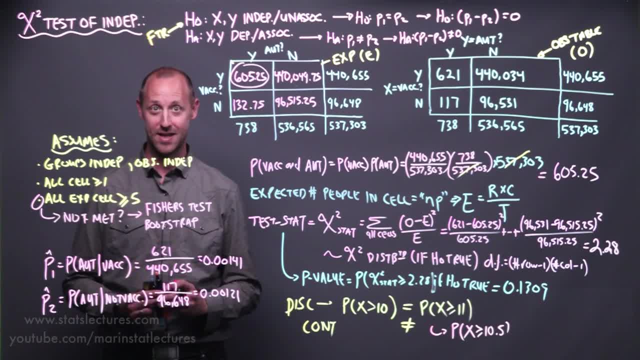 and I thought, having this platform, I think it's important for me to to say something here. recently, there's been this kind of wave of anti-vaxxers, or people being anti-vaccination, and I thought it's important to say a few things here now. I'm not going to speculate on exactly. 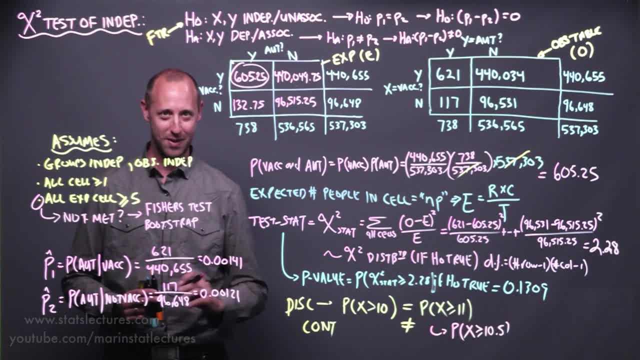 what goes on in inside people's brains or why they might be thinking this or going down this path. but I do want to make some statements about science versus non-science, and so someone who's in the anti-vaccination kind of camp. they tend to make really alarming statements like vaccination. 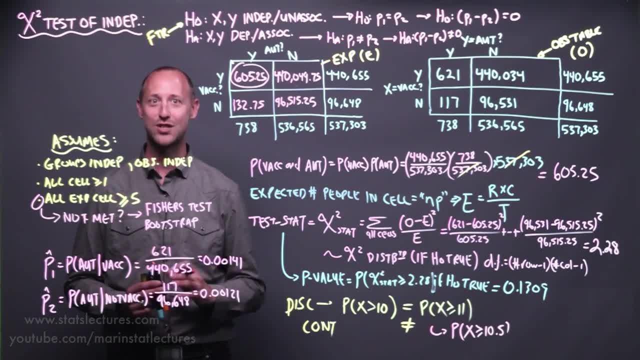 leads to autism. yeah, which sounds like a very strong statement. and then, as a scientist, what we have to say is: we don't have any evidence to believe that there's an association between vaccination and autism. okay, which sounds like a a more a weaker statement. right, we don't have any. 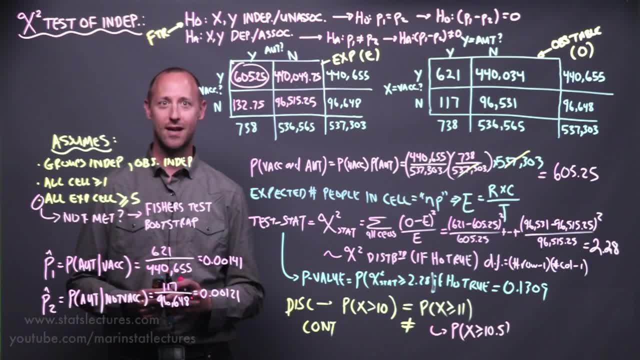 evidence, but we're not really sure about it, and the reason is that as scientists, we know it's Extremely difficult, if not impossible, to prove a null. It's very difficult to prove something doesn't happen. We always have to make statements like this that we don't have evidence to believe something's happening. 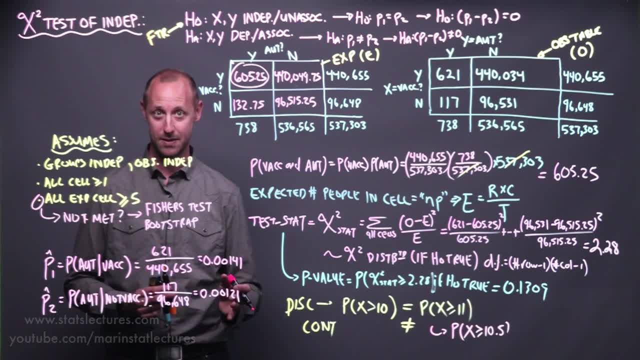 It's very difficult for us to definitively make these statements okay. so I think that's part of the problem is that these alarmists make these really bold sounding statements and Scientists make these statements that sound weaker, like oh, we don't really know and we're not sure, and that's not really the case. 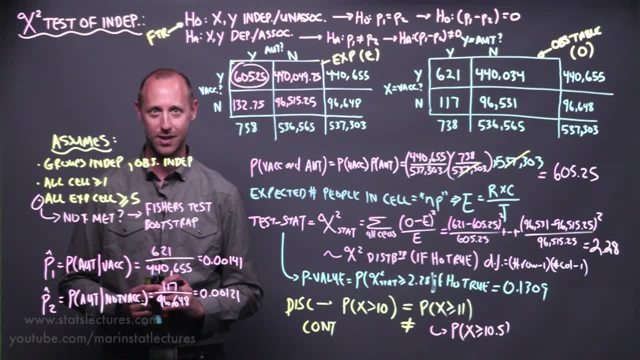 I mean. the case is that we don't have any evidence to suggest that they're associated, But it's nearly impossible for us to say that they are not associated. Where all this started of was someone named Andrew Wakefield in 1998.. He published a paper linking 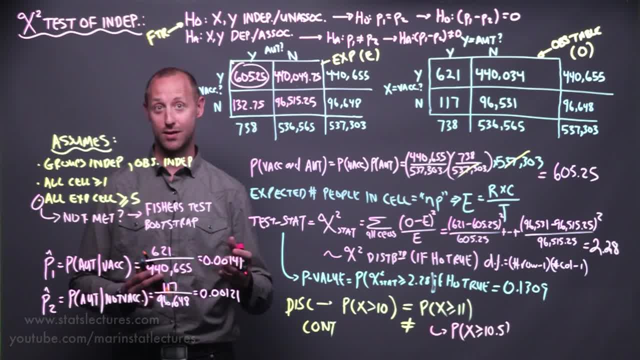 Vaccination for MMR and autism. later It was discovered. a lot of things were discovered. There were some huge conflicts of interest with him. It was found that the data was falsified, meaning the data was changed To make it look like there was an association when there's not. 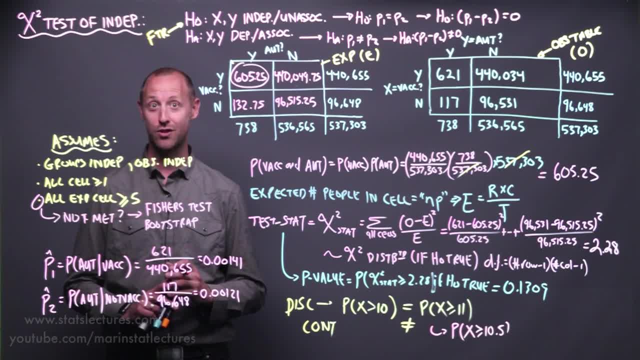 The paper was retracted. This was published in the New England Journal of Medicine. It was actually pulled out of publication. They said that this paper is falsified. It's wrong person manipulated the data and they removed it. Andrew Wakefield also had his license removed and meaning they they're not letting him practice as a doctor anymore. 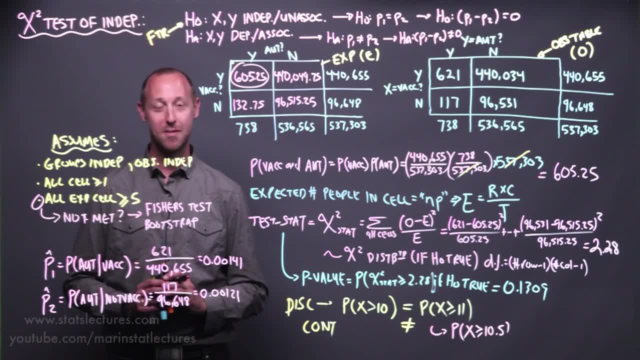 but this kind of falsified paper did a lot of damage and it still lives on and it still gets cited as a as a You know a paper to say that the two are related, when it's completely falsified. Thanks for watching our video. subscribe to our channel. 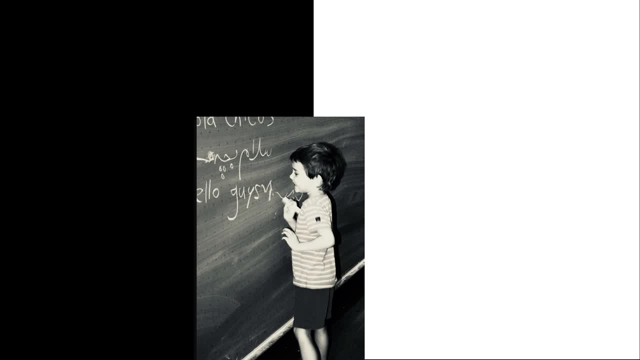 share our videos. Stick around, guys, cuz we got lots more Statistics. is hard to say, Poopally. 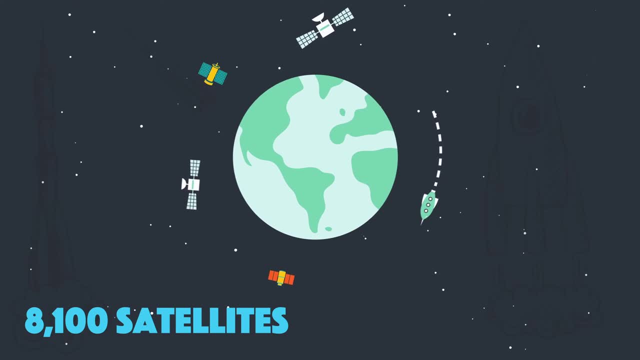 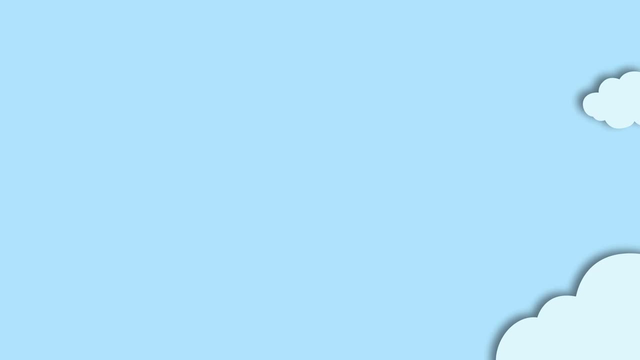 What is aerospace engineering? With 8,100 satellites and nearly 25,000 aircraft flying around the world, you know the role of an aerospace engineer is something quite special. So at the core, an aerospace engineer would design something to fly. We're talking aircraft. 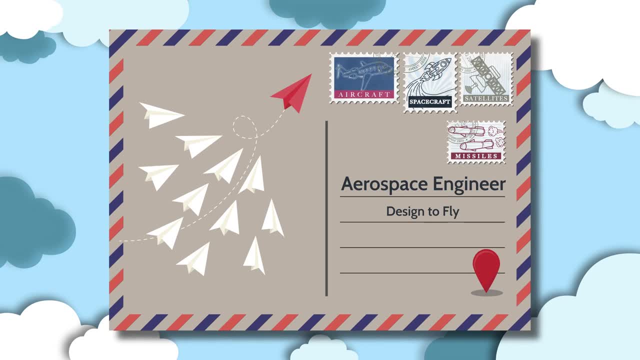 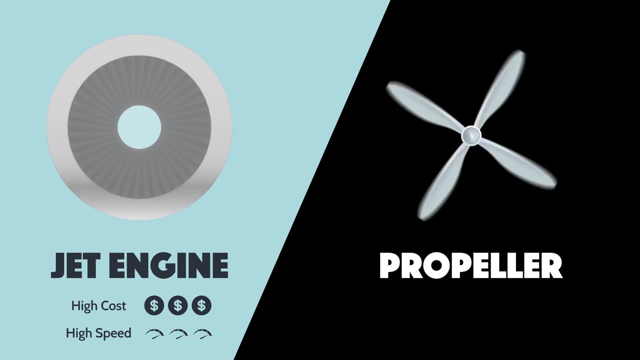 spacecraft, satellites, missiles, Yeah that kind of stuff. Now, how it intends on flying is where it gets interesting. I mean, is the craft going to use jet engines or propellers? What's about the fuel? Are we going for the classic kerosene? 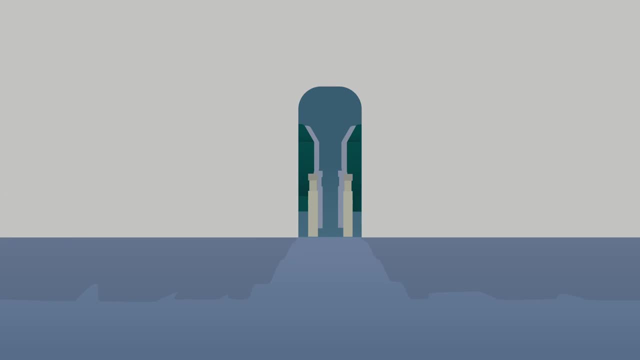 or thinking solar panels and batteries. What's about the passengers? How many? Is it over 500, or are we just flying for one that specializes in air-to-air combat? And the range of the craft? Are we traveling over 100 million miles? 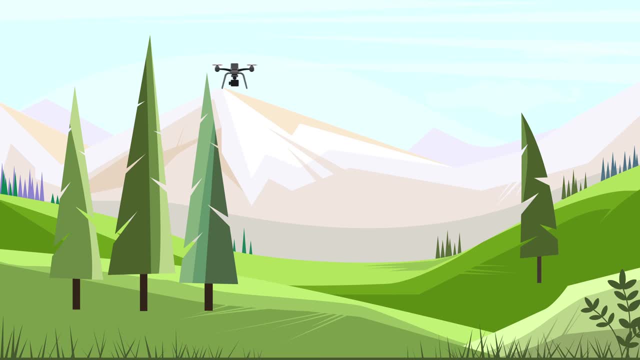 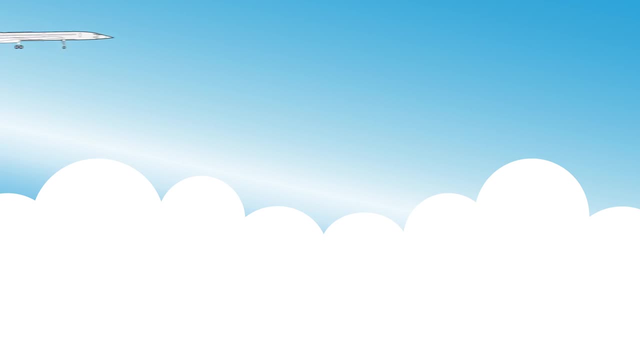 or is it just over the ridge to get those breathtaking drone shots? These are the questions that engineers need to answer before any component is designed. Let's take the Concorde, for example, Now. for those of you who don't know, it was the fastest commercial plane to take the skies. 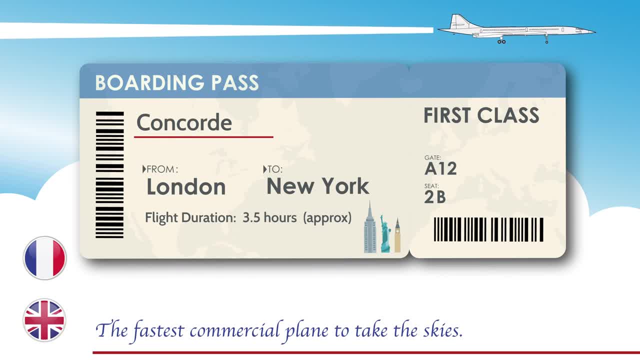 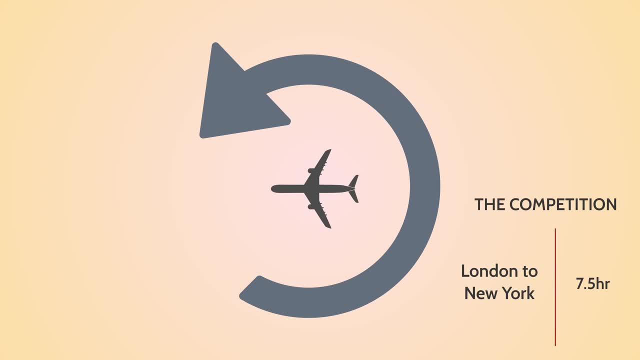 reducing the London to New York flight duration to just three hours. It was at the very edge of engineering. Some would even say it was the Bugatti Veyron of the skies. But how can engineers just casually reduce the flight time by over half? 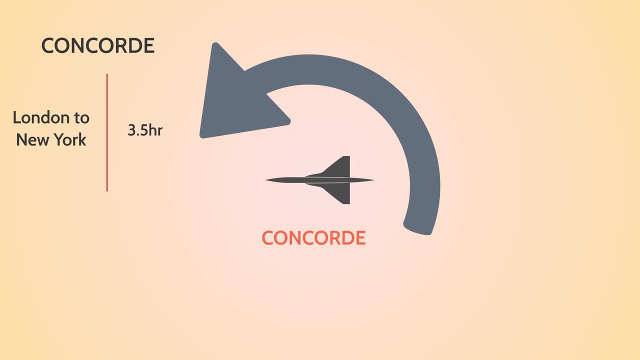 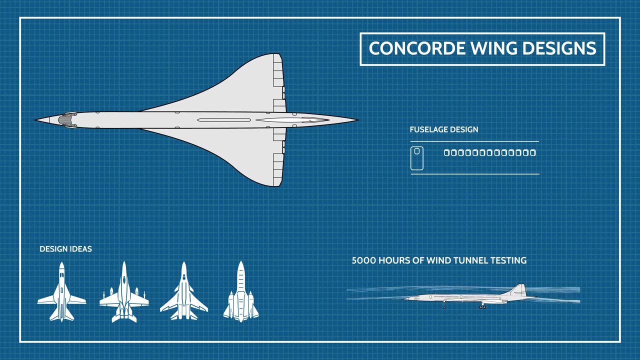 Well, they're going to have to go all out designing from the ground up. First, let's take the wings. The design concept for them were taken from fighter jets. Add the fuselage and another 5,000 hours of wind tunnel testing and you have. 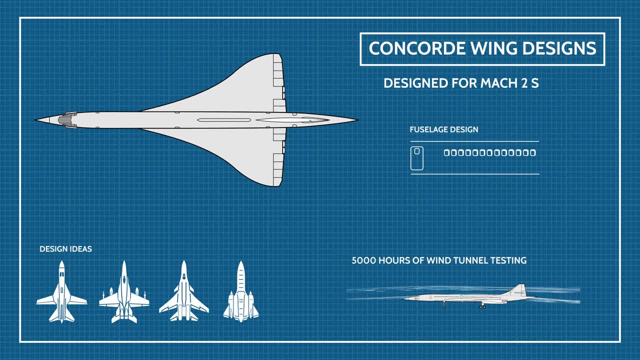 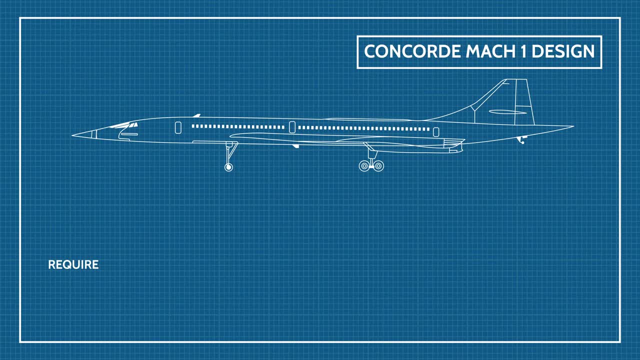 just the shape of the Concorde. But wait, that shape is for Mach 2 speeds when flying. What about takeoff and landing? Not only are the drag coefficients completely different here, but the pilot actually needs to see the runway. So what did the aerospace engineers do?